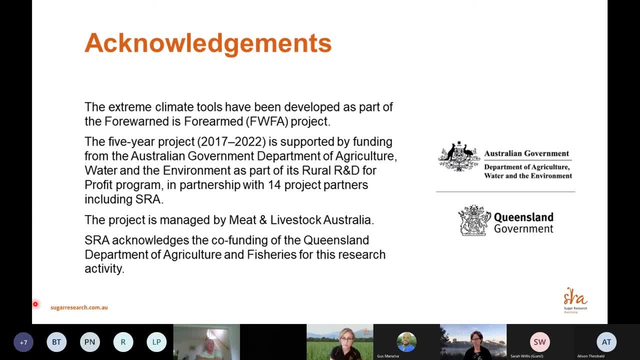 A key component of Debbie's work is leading research and development projects and interacting with stakeholders. Debbie has a PhD in climatology and has been at the Bureau for nearly 20 years. Debbie, thanks so much for joining us, And over to you. 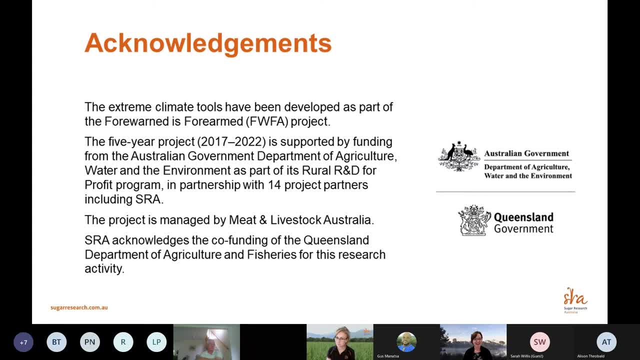 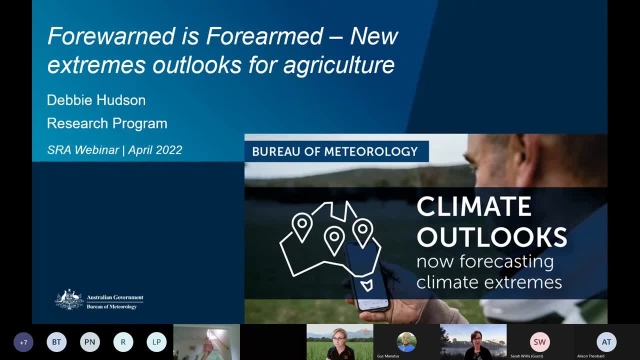 Thanks very much, Cathy. It's really good to be here And, as Cathy said, I'm going to be presenting to you about the Forewarned Is Forwarned project, which looked to develop new outlooks focused on the agriculture sector. 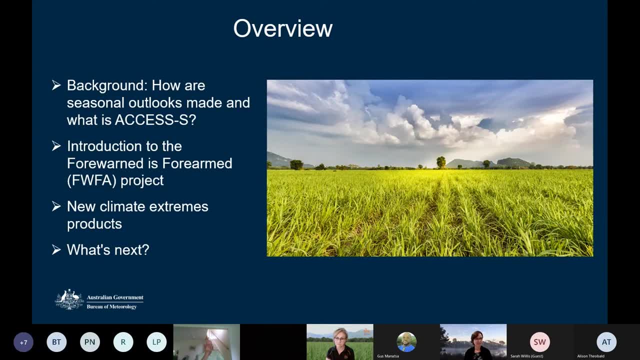 But before I do that, I'm going to give you a little bit of a background into how seasonal outlooks are actually made and what Access S is. And I'm going to give you a little bit of a background into how seasonal outlooks are actually made and what Access S is. 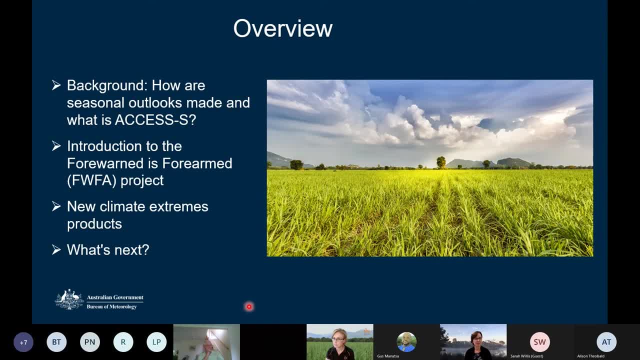 And I'm going to give you a little bit of a background into how seasonal outlooks are actually made and what Access S is. Then I'll introduce the project to you and then talk a bit about some of the new forecasts that are available and what's coming next. 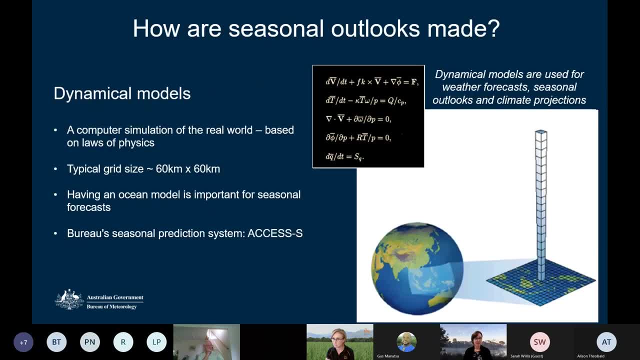 Then I'll introduce the project to you and then talk a bit about some of the new forecasts that are available and what's coming next. So, first of all, how do we actually make seasonal forecasts? So for seasonal forecasts, we use the same kind of models that give you your weather forecasts, and they're what we call dynamical models. 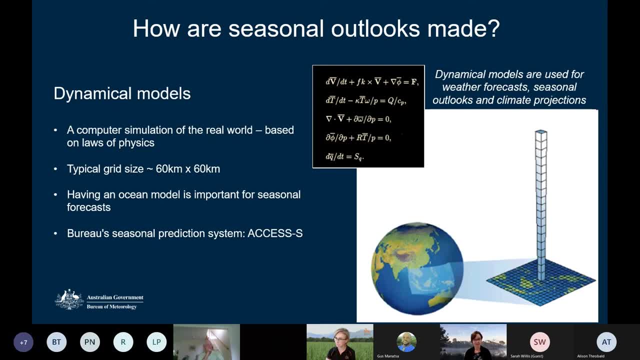 because they're based on the equations of physics. So they're based on things that you know the way we know that say heat. So they're based on things that you know the way we know that, saying heat and moisture are transferred within the atmosphere. 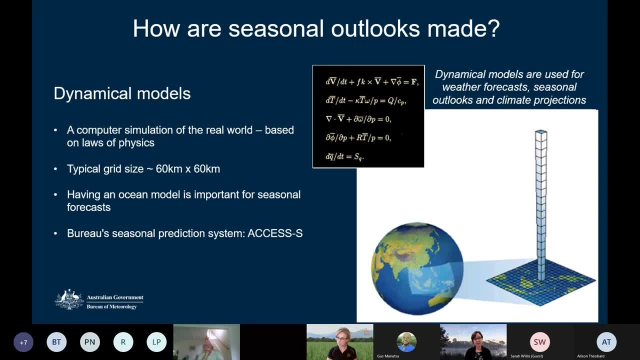 and between the atmosphere and the land surface, And so really it's like a computer simulation of the real world, And what happens is that the globe is broken up into grid boxes and, in a seasonal forecast model, the grid box typically has a resolution of about 60 kilometres by 60 kilometres. 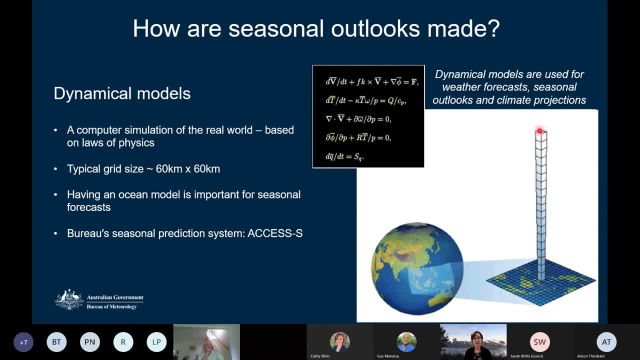 But then we also model what's happening up into the atmosphere. So we have layers that go up into the atmosphere And for seasonal prediction having an ocean model is very important, So we also model what's going on in the ocean. Now the Bureau's seasonal prediction system is what we call Axis S. 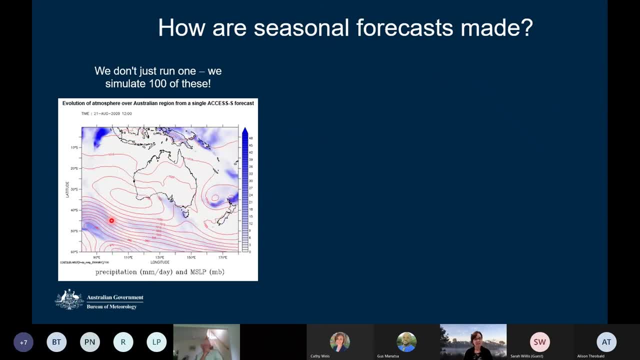 And so this animation that you can see here is actually the output from one forecast run with Axis S, And it's showing how it's simulating the weather day by day, just like the models. They produce the weather forecast, And here you can see the lines are pressure. 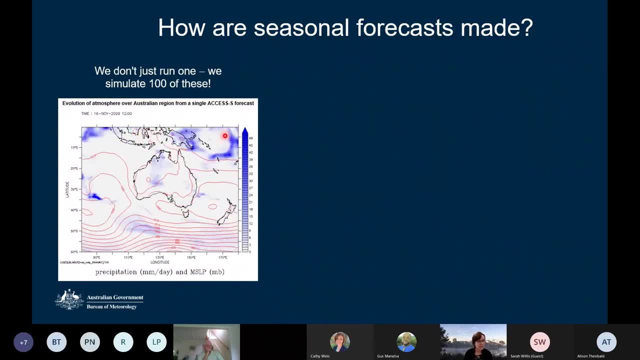 and the shaded blue areas is rainfall And you can see features like tropical- all those that will be tropical cycling that's going to come along here soon. Yep, there it comes. So the model is simulating what's going on in the atmosphere every single day. 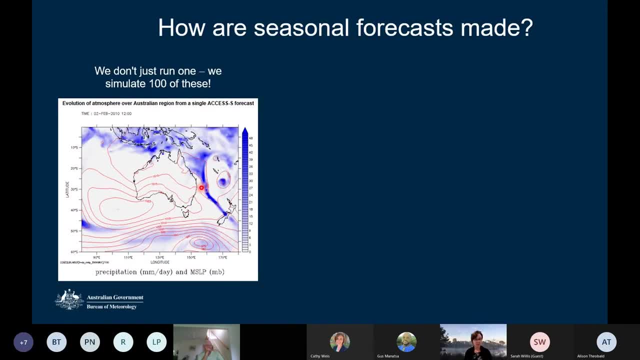 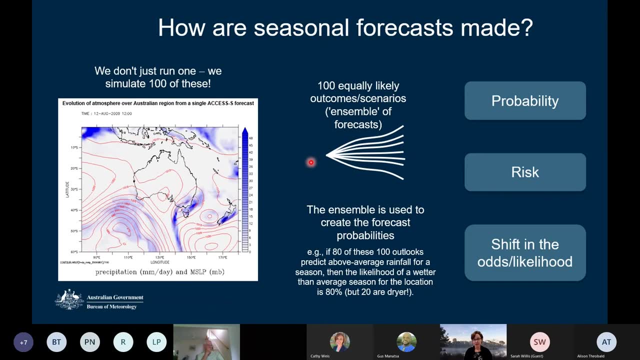 But there's uncertainty in how the weather will evolve And because of that, we don't just run one of those, We actually run 100. And so we're running, you know, 100 plausible scenarios or outcomes, And that's actually what we use to provide the probabilities. 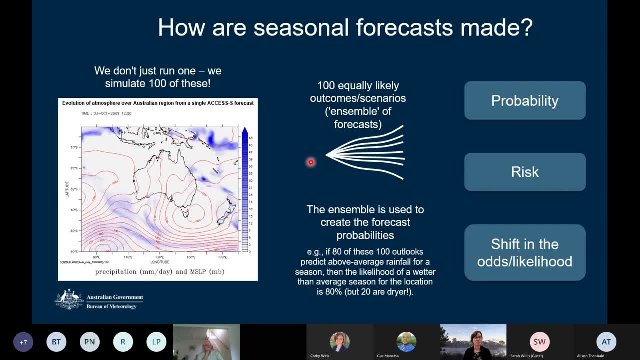 that you see when you look at the seasonal outlooks. So, for example, if 80 of those 100 outlooks predict above average rainfall for a given season in your area, then it's basically saying 80 of those are suggesting that it's going to be wetter than average. 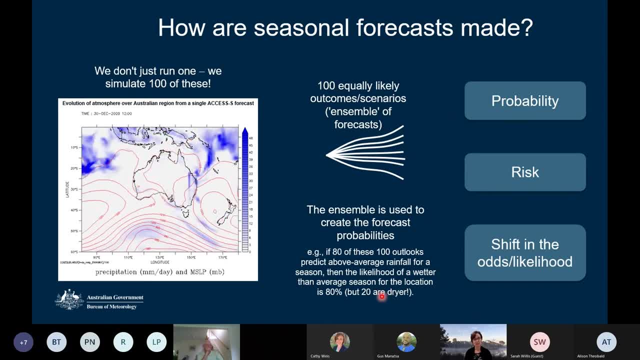 But remember that 20 of them also said it would be drier. So I think that the key thing with seasonal forecasting is that you know, although users or everybody wants to know exactly what's going to happen, you know people want to know: is it going to be dry or is it going to be wet? 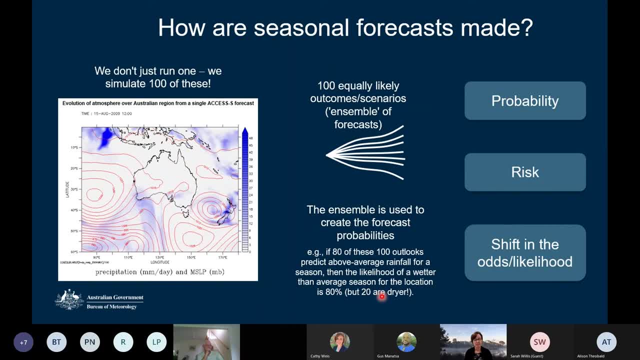 But really it's more about probability and risk and shifts in the odds. So you know how are the odds stacking in one direction or the other, And so it's taking this full information rather than using a single outcome. Okay, So just to give you a little bit of background, what a forecast system is. 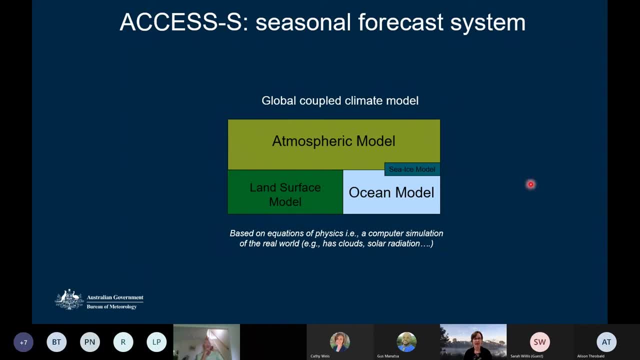 So XSS, as I said, is the Bureau's seasonal forecast system And at the core of it is a model, And it's what we call a coupled model, which means that it's got an atmospheric model coupled to an ocean model, But there's also a land surface model and a sea ice model. 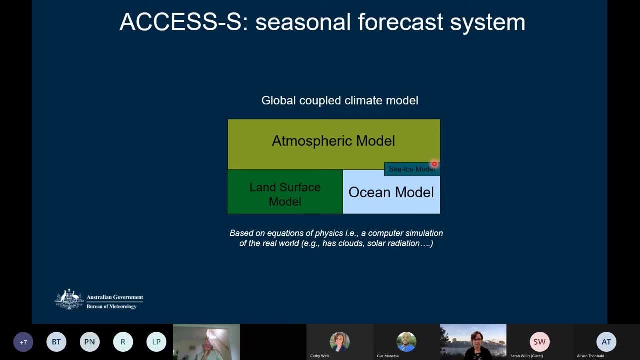 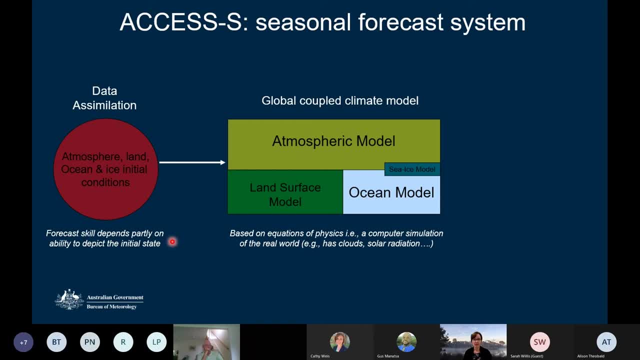 Okay, So we actually need more than just the model When we run a forecast. we actually need to be able to start the forecast with our best estimate of what the current state of the atmosphere, ocean and land is now, And so we get all the latest observations that we can from like ships and satellites. 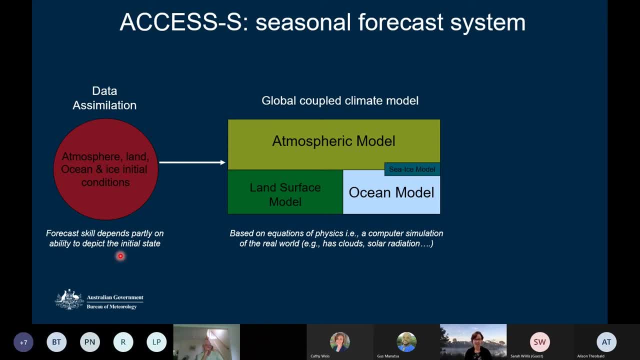 and ground stations to get a picture of what the land and the atmosphere is. And this process of getting the observations and putting them into the model for the start of the forecast is what we call data simulation, And that process is actually almost as complicated as the model itself. 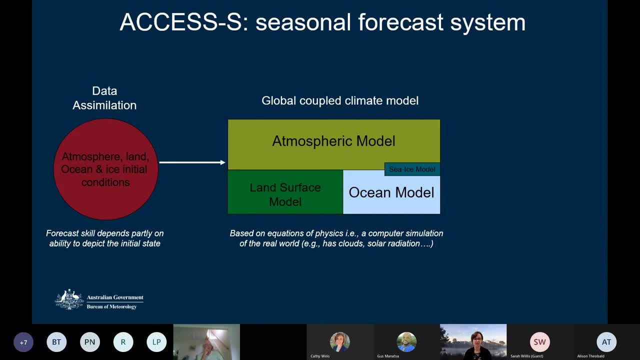 And so then, once we have that initial starting point, the model can then freely evolve, like you saw in that animation, to create the forecast. But, as I showed previously, we don't just run one, we run a multiple, because we need to take into account that you know, there's uncertainties in the way that the weather 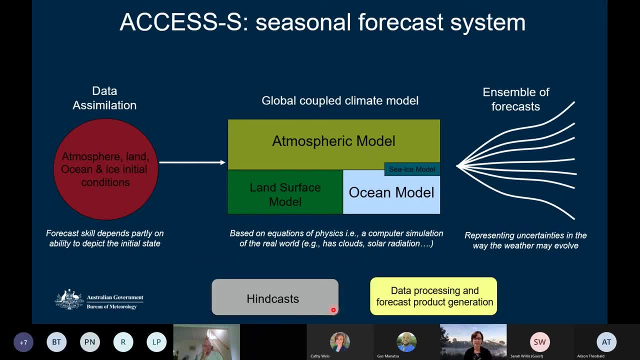 can evolve. And then the other thing in seasonal prediction is we run a set of forecasts for a period retrospectively in the past, which we call a hindcast, And usually that's about a 30 year period. And the reason we do that is we want to. we use that to look at how good the system is. 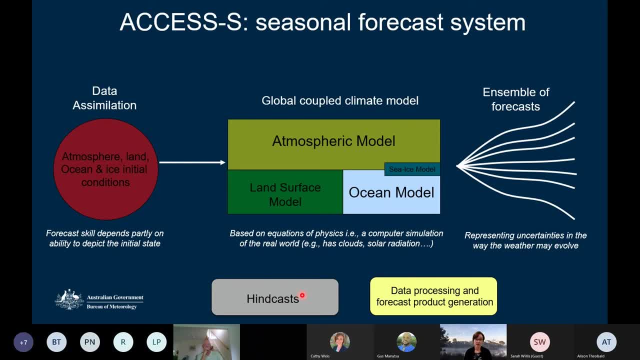 What is the skill of the system? And we also use it to calibrate the forecast that we issue in real time. And, of course, we have to process the output from the model to produce the kind of forecast that you see on our web pages for forecasts of El Nino or Australian climate. So really, XSS is a model that we use to predict what the weather is going to look like in the future. So really, XSS is a model that we use to predict what the weather is going to look like in the future. So really, XSS is a model that we use to predict what the weather is going to look like in the future. 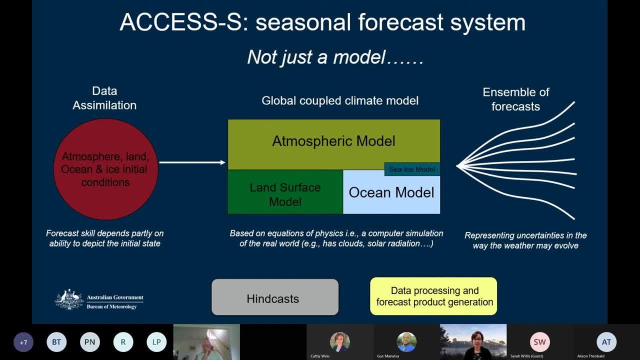 So really, XSS is more than just a model. So really XSS is a model that we use to predict what the weather is going to look like in the future. Now we've just had a major upgrade to our seasonal prediction system from XSS Version. 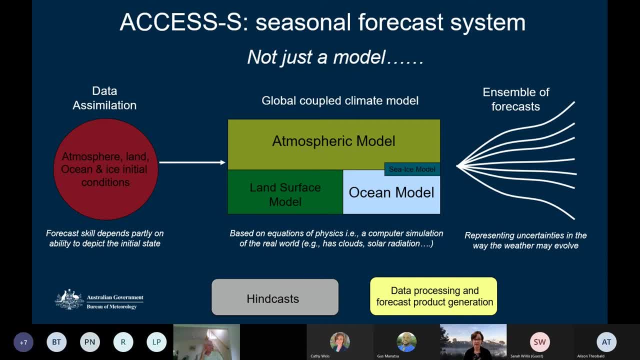 1 to Version 2.. And the main changes that we made in the system were actually in this data simulation, part of getting the starting conditions for the model and changing the data are possible. males in can actually have a very big impact on the forecast. 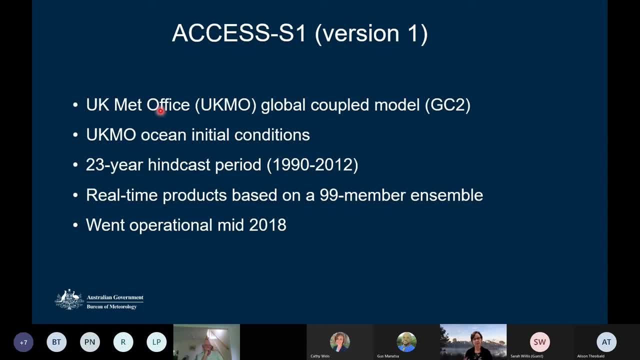 So XSS version one. So the development of our seasonal prediction system is a collaboration with NASA and NASA studies. region software is a collaboration with the uk meteorological office and we use their model and in version one we also use their ocean starting conditions. we ran our retrospective forecasts over a 23-year. 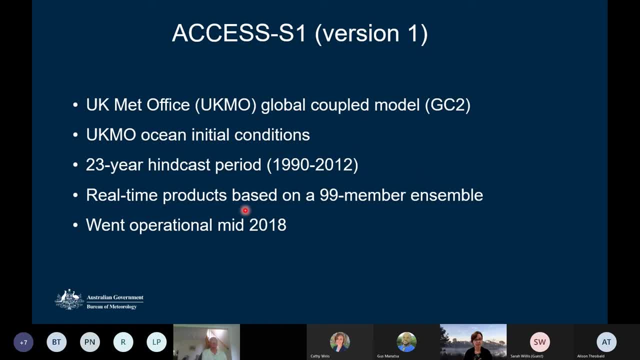 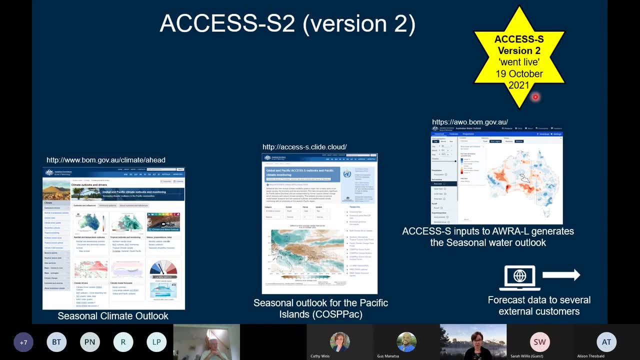 period and access s1 has been was running since the middle of 2018.. but now access version 2 went live in october last year and access s supports several services. the one you're probably most familiar with is our, obviously our seasonal climate outlook, but we also provide outputs. 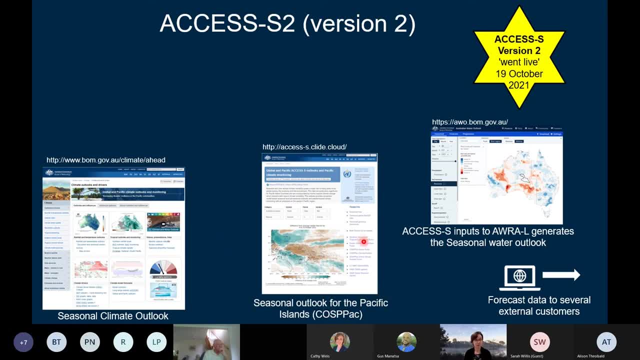 for the pacific islands and and actually global outlooks. we also are the. the output from our access s also goes feeds into a water balance model and produces seasonal forecasts of soil moisture and runoff, and this is a relatively new product at the bureau, um. so yeah, maybe you want to go and explore that and look at what some of the outputs for. 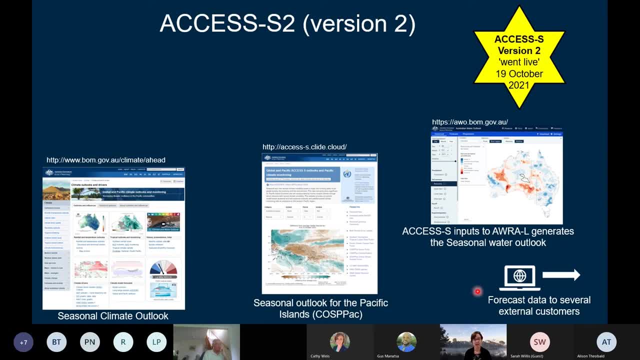 soil, moisture and runoff and and also evapotranspiration, and then we also serve data to external customers. so, as i said before, the main difference between s1 and s2 is that in s2 we actually do our own data simulation, we produce our own initial states. um, that has 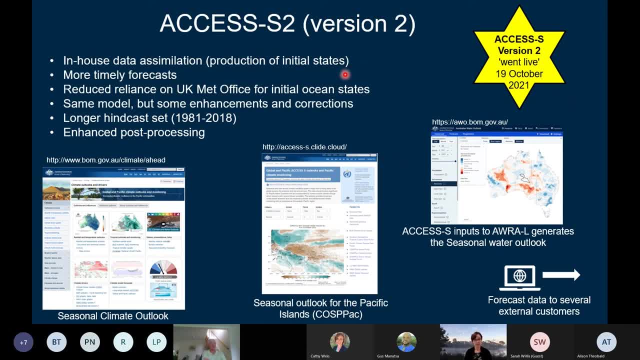 an implication that we can actually do it um. we can actually create the forecasts um faster, more readily, which means that they um actually more accurate, um more timely, um. it means we have less reliance on the med office. um. the model is pretty much the same in access s2, but what we've 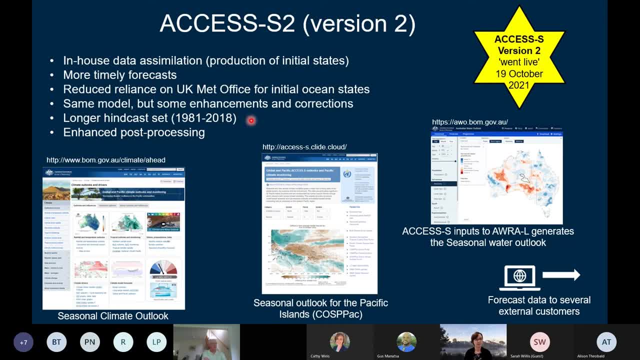 also done is we've done a larger test period over the past, and that's actually really valuable because it helps us to get more um robust estimates of the system's performance and it's also better for our calibration. so i'm just going to show you two things. 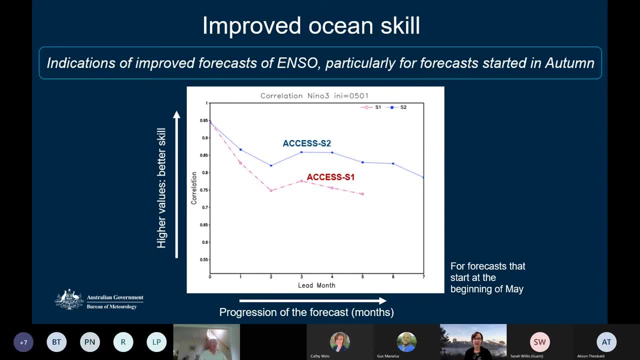 about the improvement. so in access s2 it looks like we've actually got better ocean initial states than we had in in access s1, and that actually improves our forecasts of el nino and lanier, especially during autumn, and so what this graph here shows is correlation skills. 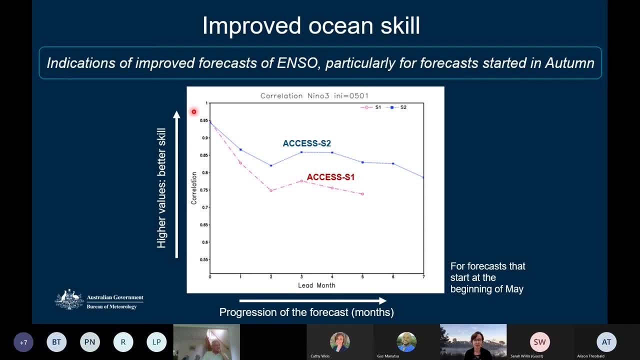 so on the y-axis is correlation, so higher values are better um, and it's showing the correlation for um, nino3, sea surface temperature anomalies, which is which is indicator of of el nino and la nina. and then on the y-axis, on the x-axis is the progression of 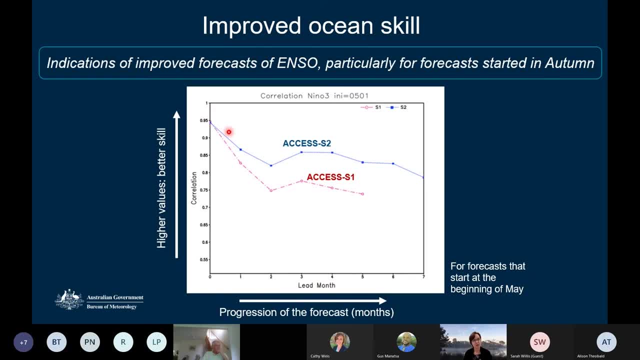 the forecast in months. so as you go out in the forecast the skill or the correlation decreases. but you'll see that in access s2 that skill is decreasing less rapidly. so the skill is better in access s2 compared to axis s1. and this is really good for this time of year because 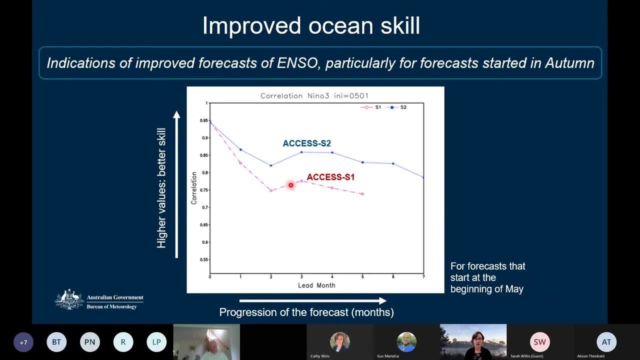 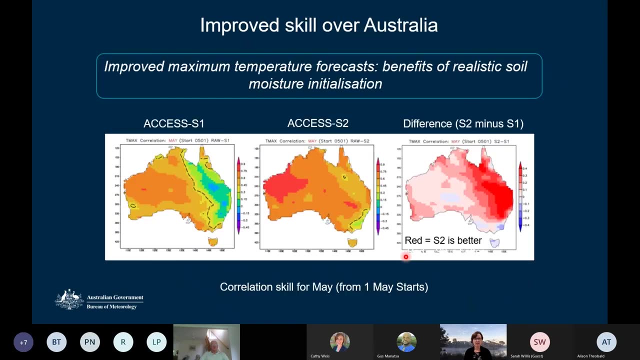 forecasts that start around now and in may in autumn- really challenging time of year for forecasts, and all international models experience um difficulty predicting um in so this time of year, so that's a really pleasing result. the other thing that we've improved is um the starting conditions for soil moisture. 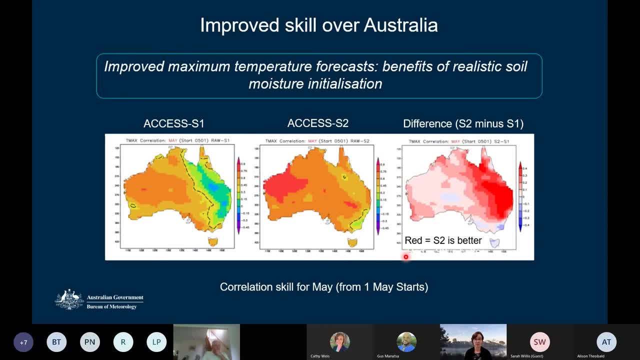 in in the forecast in access s2, and we've made that more realistic and that's actually made a big difference for our accuracy of our maximum temperature forecasts. so what these maps show is this is forecast um in the forecast starting in may um and the skill that you get for may for access s1, access. 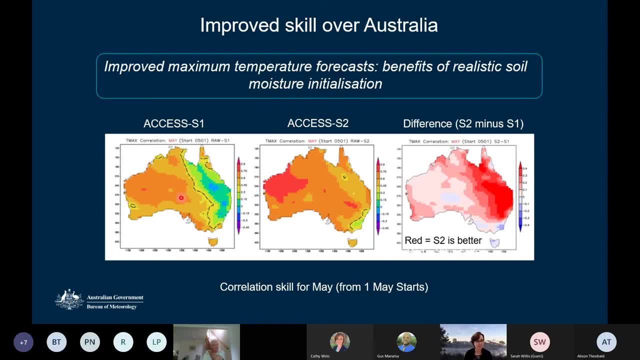 s2 and the difference, and so in in these two the warmer colors indicate better skill and in this one is showing the difference. so the access s2 skill um minus s1 skill, so red is better. so you can see that there's a significant improvement in the skill over eastern and um australia. well, 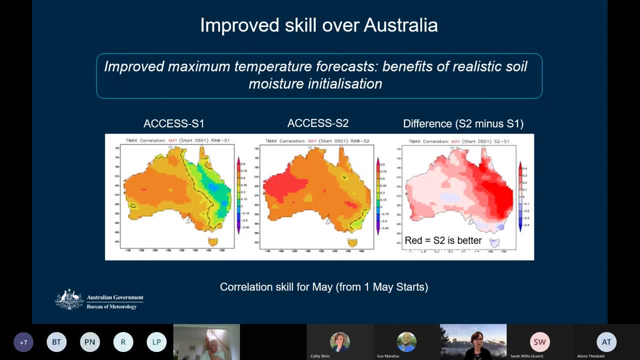 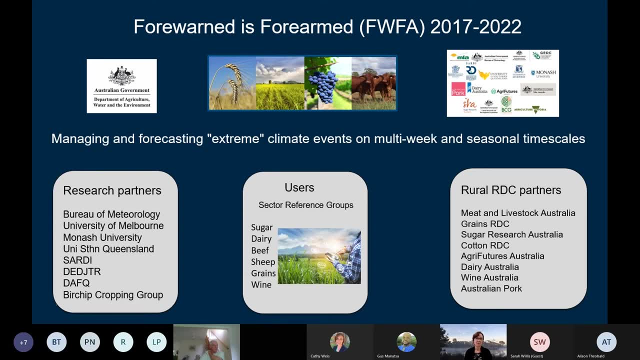 over most of australia, but particularly over eastern regions. you know, we got the CWI um real estate a little bit more obviously. it's a little bit less stringent, especially for urban areas, and so we've been trying to do that and with this question i've been able to see that you know what the differences are between the um. 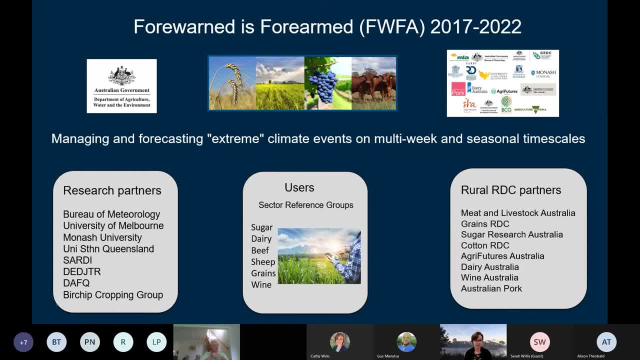 on the sql and then the sql map um, between the sql map and for the sql map um. i've got a couple of slides that i've been able to follow, so i'm going to go through a little bit of a list. what is the chance you can have above or below median conditions? 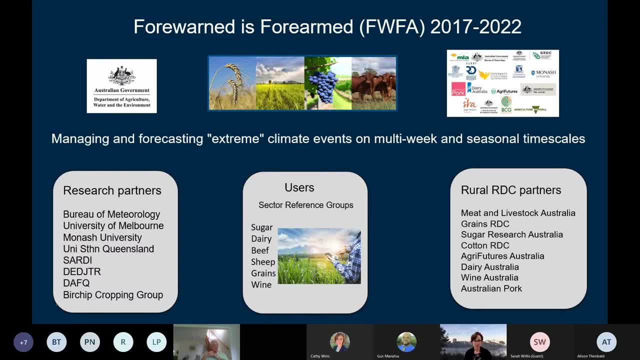 And so in this project we've got multiple research partners- you can see here who are experts in different agricultural sectors- And we also have funding and involvement from several RDCs, including Sugar Research Australia, And a key aspect of the project has been users. 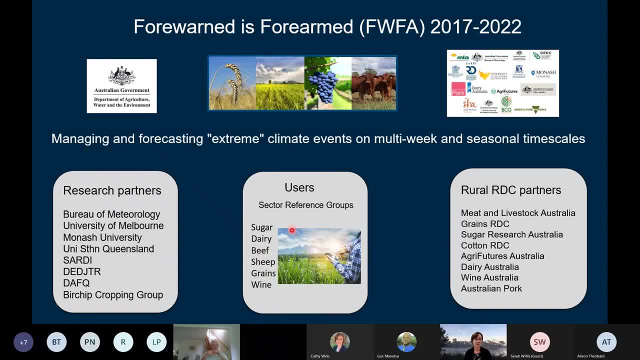 They've played a really critical role and we've had different. we've had reference groups for the key sectors that have funded the project, including a sugar reference group, And our sugar reference group was run by the University of Southern Queensland and DAF Q. 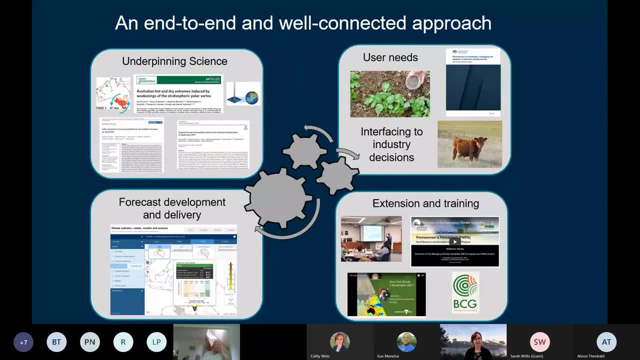 So one of the things that I think makes the project exciting is that it actually encompasses an end to end approach, And I think that really has increased its effectiveness. So it's included: underpinning science, Forecast development and delivery, engagement with users. how to interface forecasts to industry decisions. 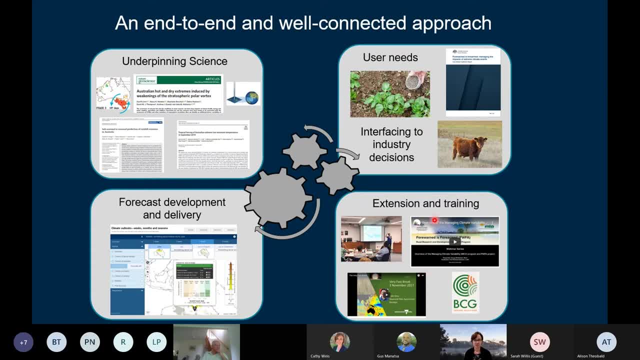 and ultimately, the, the delivery and extension of a new service, And, of course, we've had throughout the project. what's been really good is we've had interactions and feedbacks between all of these components. So, as I mentioned before, our project partners have been the ones 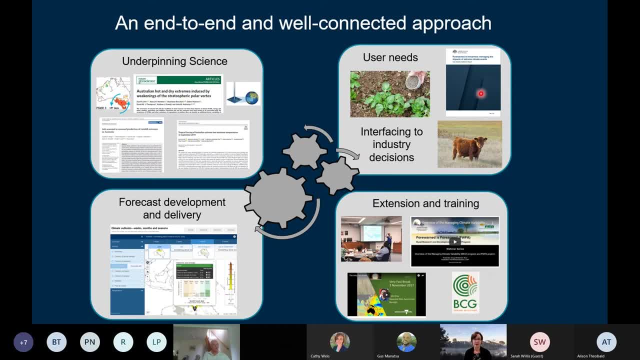 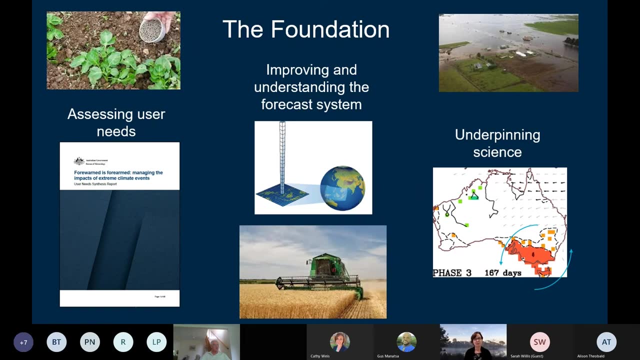 leading this interfacing to industry decisions and the development of risk management strategies. So in the case of sugar, that's been USQ and DAF and Q. So when we develop new output products, it's pretty much based on a foundation, And that foundation I like to think of is is basically understanding. 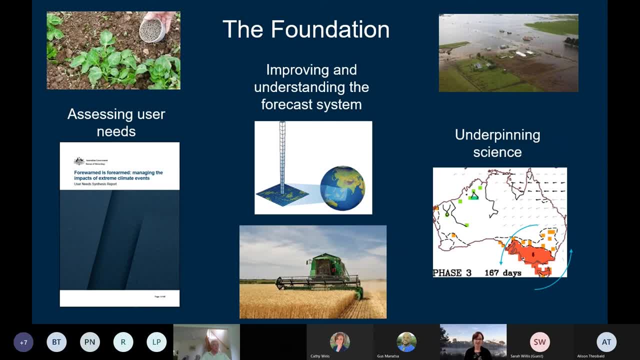 the user needs and also sort of the underpinning science. So at the start of the project we had a series of workshops and with each of the sectors involved in the project, And those workshops were aimed at understanding you know what are the main weather and climate risks. 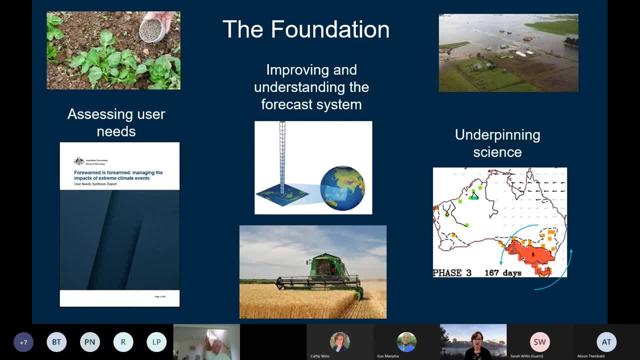 What are your main pain points? What are your key decisions? How might a forecast help you? What action might you take if you had a forecast And you know how far in advance do you need to know? And this type of information and feedback has been ongoing through the project. 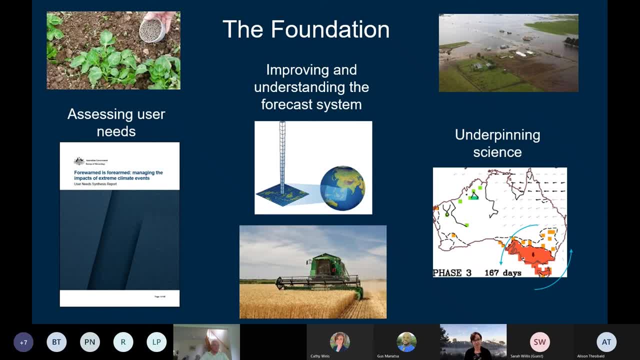 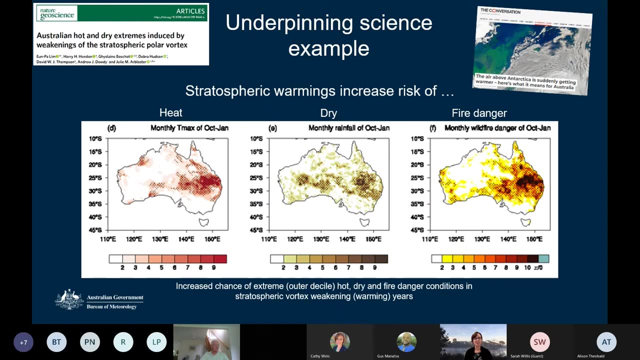 And you'll hear a little bit more about this from a sugar production perspective at the webinar on Friday with Robert Quirk and Tom Bardich. But the big component is the underpinning science. I'm just going to give you one example. So this is one piece of work that's come out of the project. 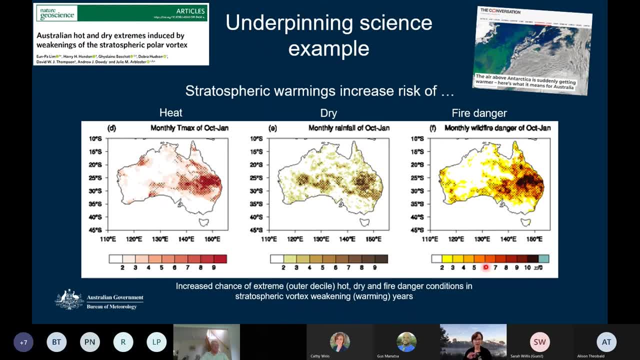 And basically it's it's. it's pretty amazing because what goes on way up in the stratosphere above Antarctica can actually have an influence on the risk of us having extreme weather and climate over Australia. Basically, when the very strong winds above Antarctica in the stratosphere weaken and the air there warms. 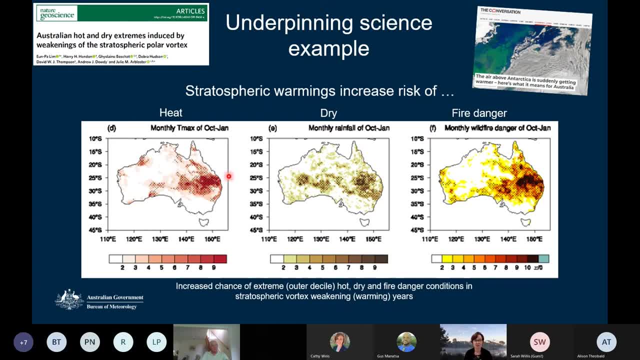 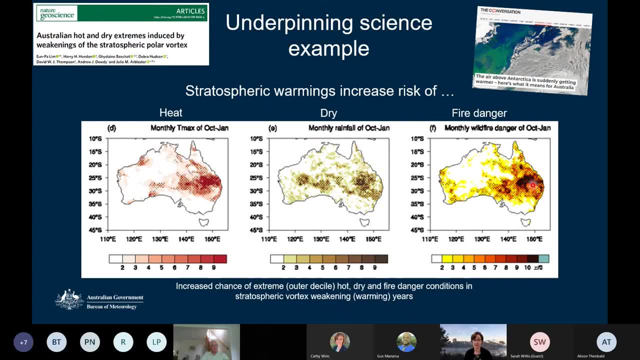 over eastern Australia and severe fire danger conditions, And the thing with this research is that all of the science that we did there actually came. it actually eventuated in 2019, when the air above Antarctica did warm unusually And we did end up having very hot and dry conditions. 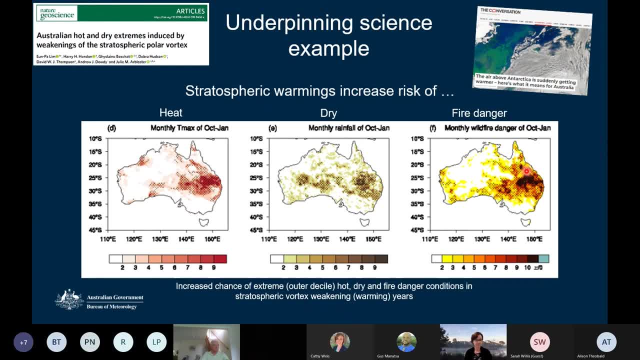 and catastrophic fire danger in spring of 2019.. And because we done this underpinning science, it actually gave us confidence in what the forecasts were saying. It gave us an understanding of what was going on, And then that impacts how we can communicate with users. 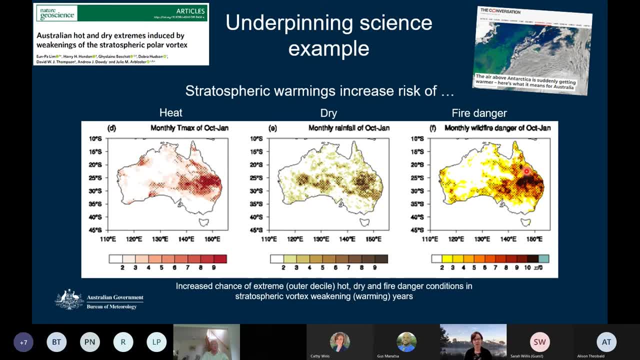 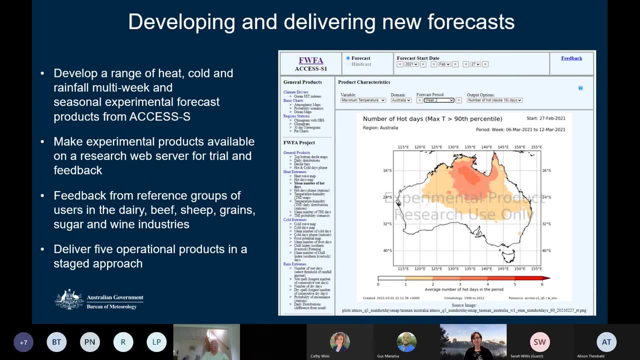 So it's very important for us to be able to be able to understand what's going on in the forecast system and how the climate variability works. OK, so now moving on to the development of the forecast product. So what we're going to do is we're going to do a little bit of research. 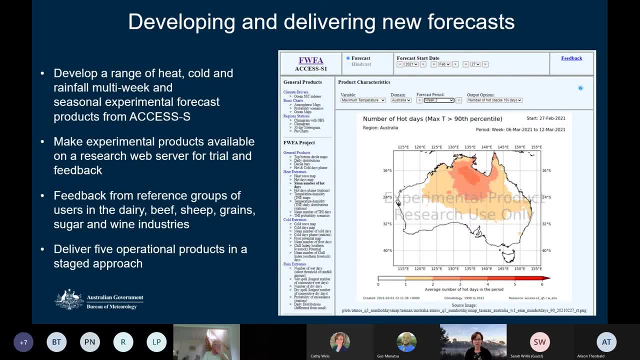 So what we're going to do is we're going to do a little bit of research. So what we did in the project is: the aim was to develop a whole range of new forecast products looking at cold, heat and rainfall- multi-week to seasonal forecasts. 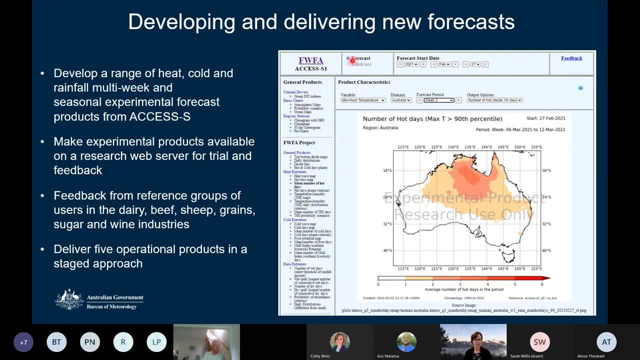 And we made them available on a research web server. You can just see a snapshot here for trial and feedback, And these forecasts were updated in real time every single day And you can see on the left hand side. here is a list of all products that we developed. 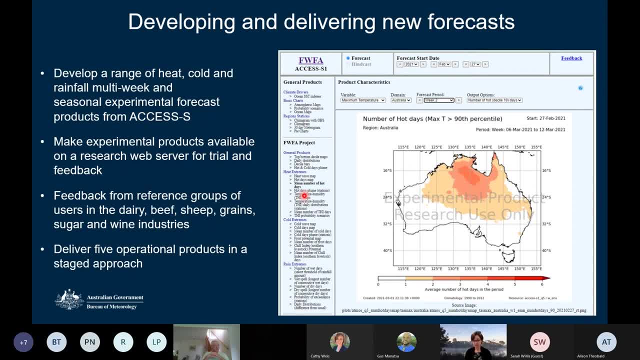 So it was a bit of a brainstorming approach, And so our users were pretty much involved in our brainstorming approach. They could see as we started adding new products, And the aim was then that we got feedback from the users And because the project has several agriculture sectors involved. 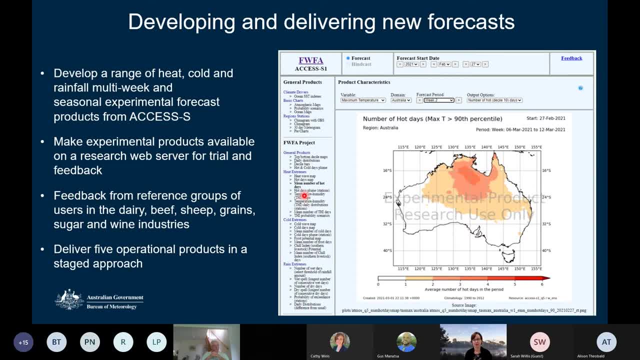 the products weren't tailored specifically to individual sectors in terms of, like you know, an index, particular index, So they were pretty generic. And so we gathered feedback from our industry reference groups on the look and feel, the interpretability, how useful the products might be. 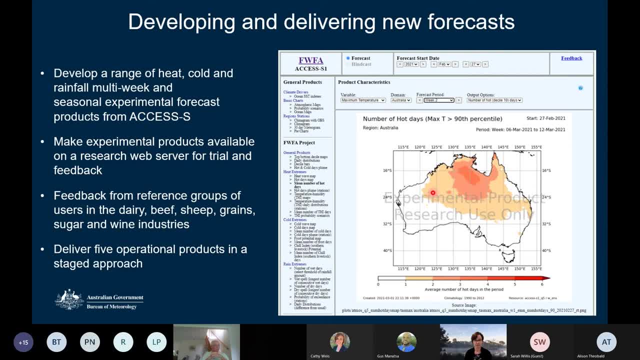 And you'll hear a bit from Robert and Tom on Friday how they used the forecasts. So really, the users have played a critical role in the development of our forecast products right from from the beginning, from the start of the project, And so from this brainstorming approach, the ultimate aim was to select. 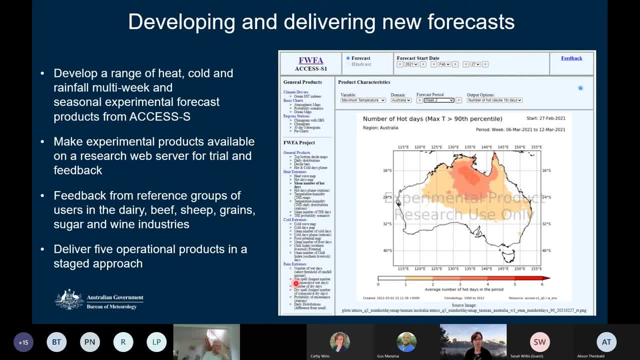 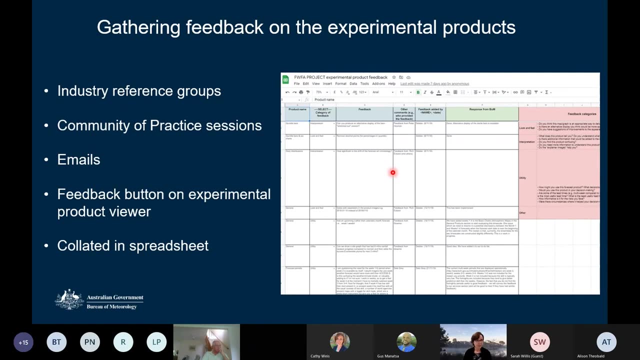 five of those products which would then appear on the Bureau's website, And we chose those five in consultation with our user groups and with the RDCs. So, and as I said, we gathered feedback from the reference groups. The project also has had a community of practice. 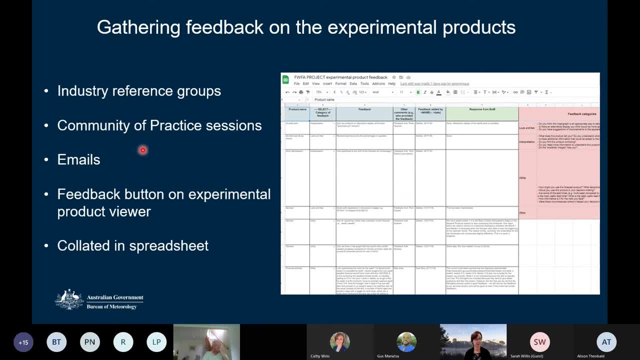 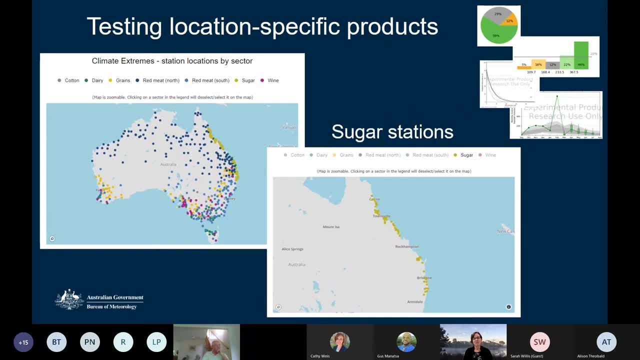 and we have a community of practice group run by the Bird Ship Copping Group, which has monthly sessions and we've collated all the feedback. So when we developed the products, so some of the products were map-based and that's fine. 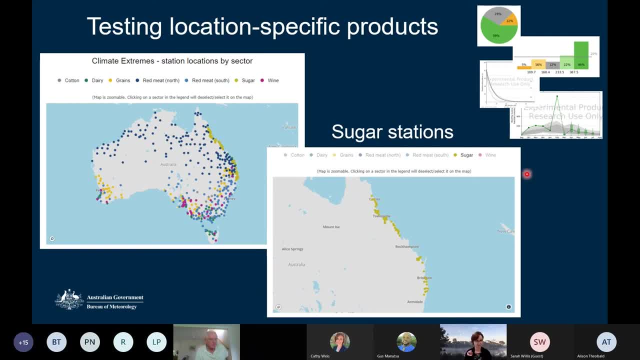 but some of the products actually were specific to a location, So you would be able to click on a location and have a product. But for our research testing, we tested it, tested these new products on about 560 locations across Australia. And for sugar, you can see the sugar stations that we had. 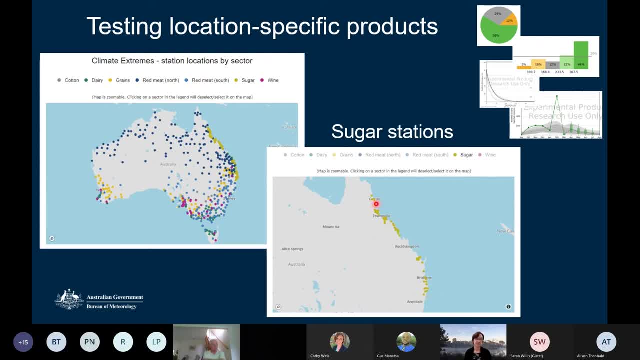 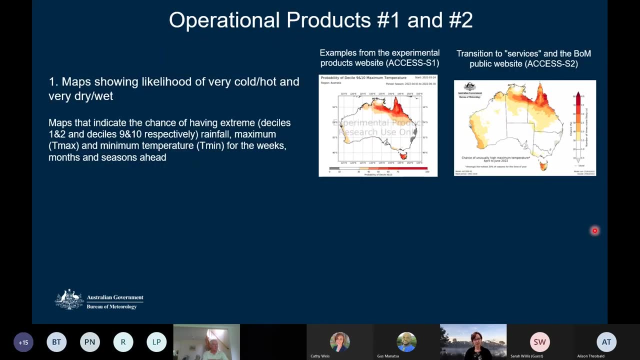 we had 80 stations, So these were stations that allow that, for which we produced forecasts that the users in our reference groups could actually go and look at forecasts for those locations. Okay, so now I'm going to talk a little bit about the actual five products. 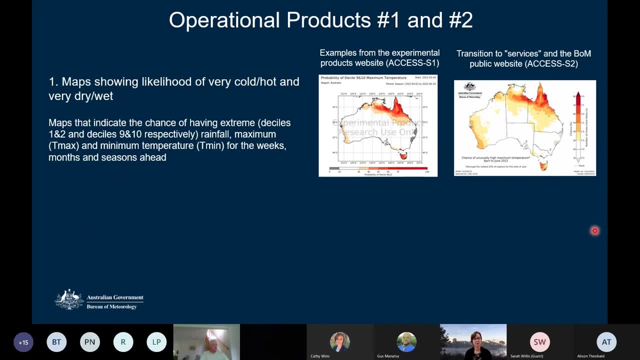 that have ended up being selected. The first two products are already operational. The first product is maps showing the chance of it actually being very hot or very cold, Or very dry and very wet, And by very we mean the top 20%. 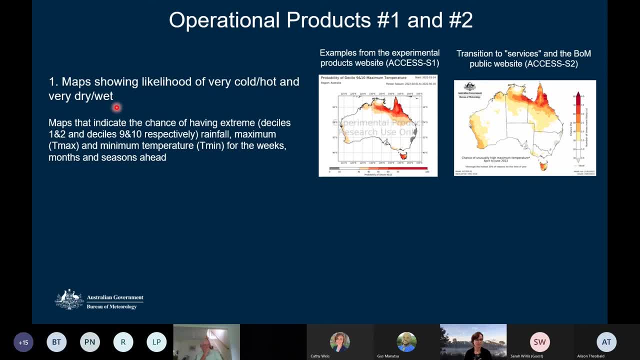 being amongst the top 20% of, say, wettest seasons, or being in the top, in the bottom 20% of driest seasons, for example, And I'll show you a little bit more about that. The other product is these bars. 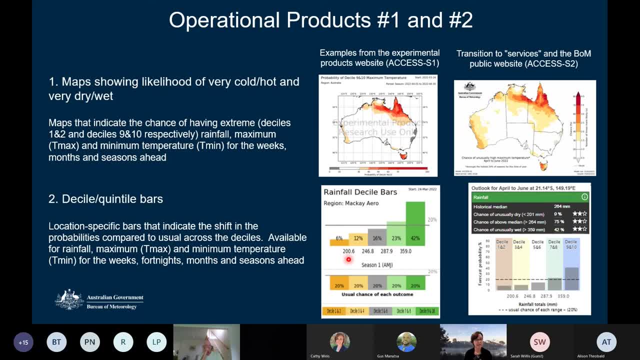 And this is an our location specific product. So I'm showing for example here Makai, And basically it's separating art into deciles. So we have the one side, decile one and two, So your driest 20%, and at the right hand side, 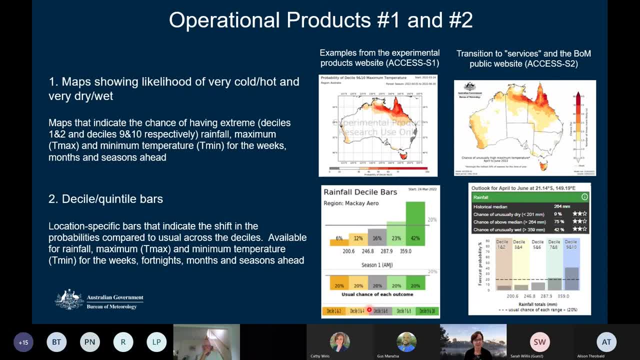 decile nine and 10. So your wettest 20%, and then the 20% categories in between, And so the usual chance of having any particular outcome in those is 20% by design. And then you look and see how the forecast shifts. 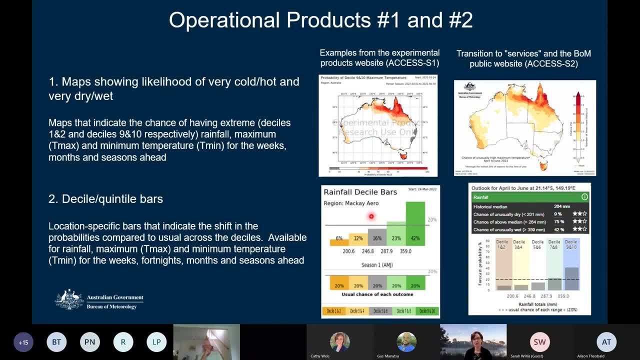 And you make those odds And I'll explain that a little bit more now. but the one thing I wanted to show you in this slide is on the left hand side, is what the product looks like in our experimental website, R&D website. 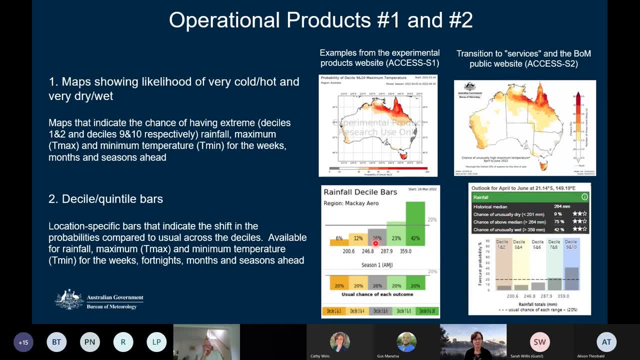 Now, because we created a whole lot of products. we didn't put a huge amount of effort into producing, you know, beautiful displays, snazzy graphics, features. But once a product, once these five products have been selected, then we've had a second round of feedback. 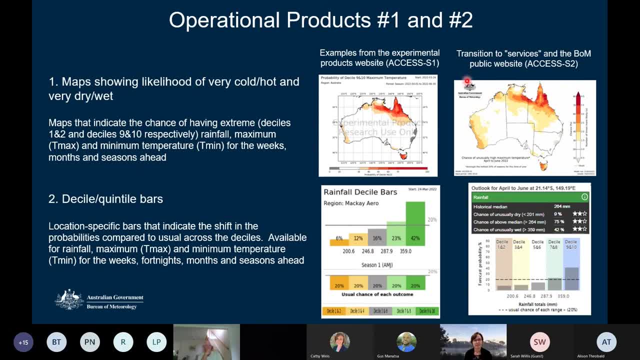 with feedback opportunities. So we've had a second round of feedback with feedback opportunities. feedback opportunities for what that product is actually going to look like and that's shown on the right hand side when it's actually displayed on the Bureau's website, where we take, you know, more attention to you know. 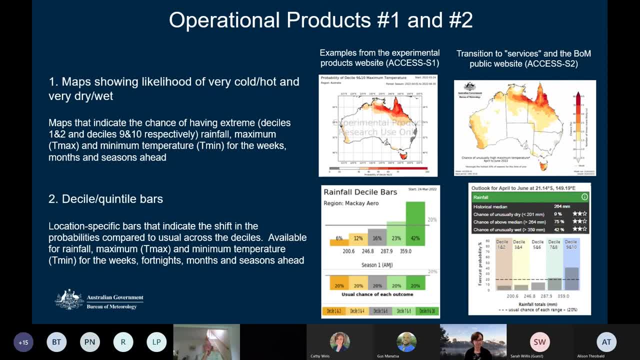 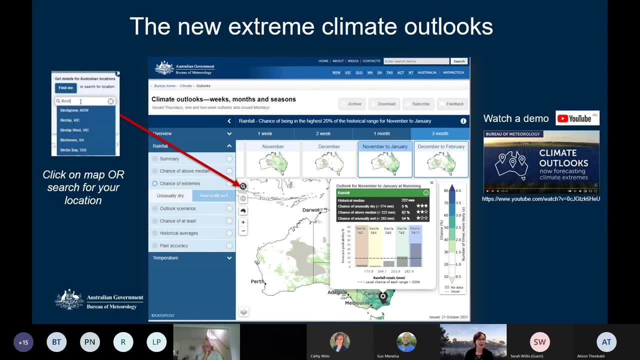 the colours that we've used, the text that's used. Okay, so the two Extreme Climate Outlook products that are available now, first of all, so you know where does it appear on the website. so hopefully you're familiar with the Climate Outlook's website and normally you would go. 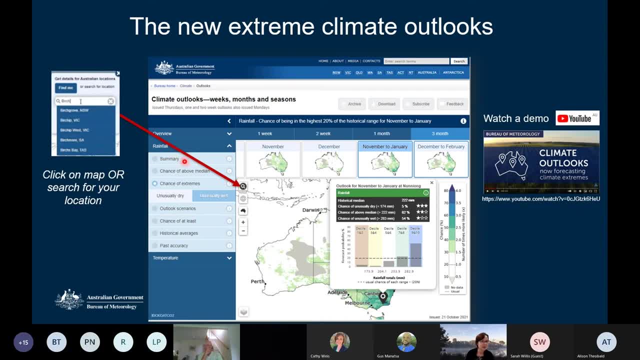 there's rainfall and temperature, so I'm just going to show here for rainfall, but the same exists for temperature and normally you would click on your sort of chance of above median For these products. there's another tab called chance of extremes. and because we're looking, 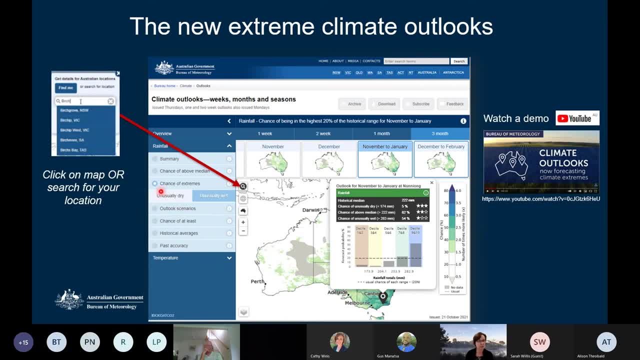 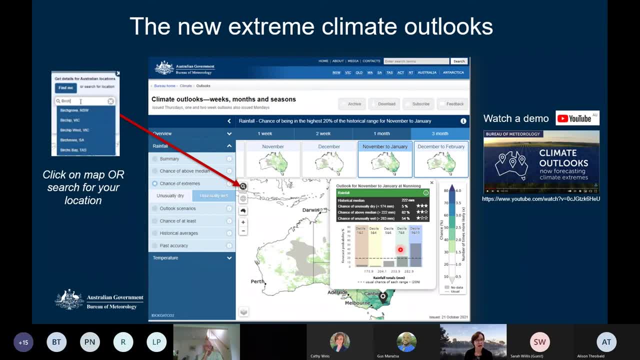 and it will come up with a location based products. A lot of users don't know this, but you don't have to click on the map, you can actually also search for your location. so if you click on that magnifying glass and you enter in your station, your location, then it will come up. 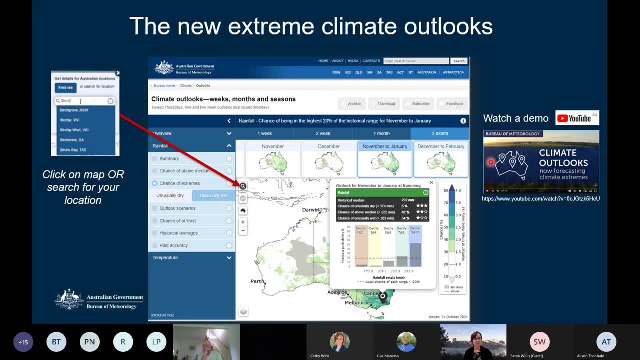 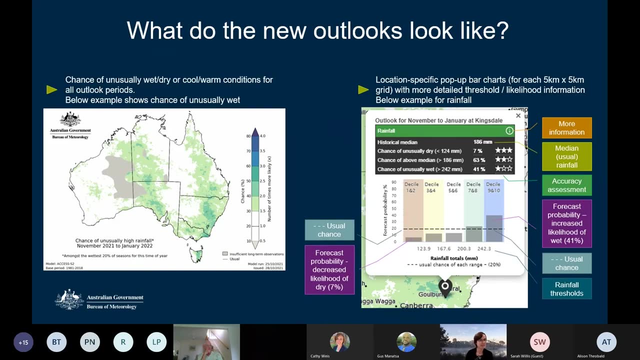 every time with your location there, and maybe later we've got this demo that shows interactively what I've just shown you here. So that's a little bit more detail about navigating the products. So now let's just look a little bit more detail at what the product is. so this is: 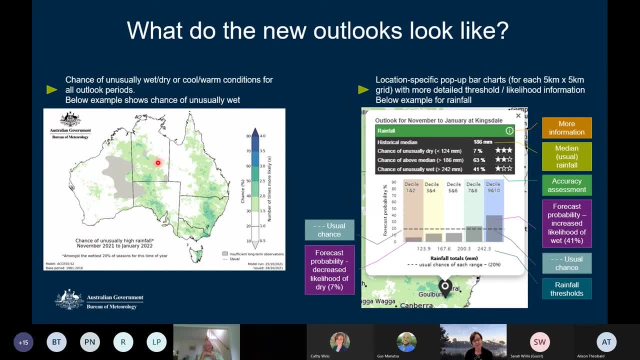 I'm showing an example for rainfall, but the same holds true if you look at maximum or minimum temperature, and so this is showing what is the chance of it being unusually high rainfall, and this example is the forecast for November to January- November last year to January this year. 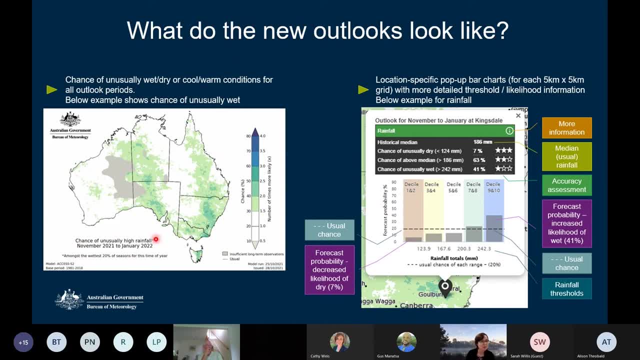 so that's three month season and by unusually wet, I've said before it's what is the chance- it's going to be amongst the wettest 20 percent of seasons that you've had for that um, that time of year. and so, um, because, because we're talking about 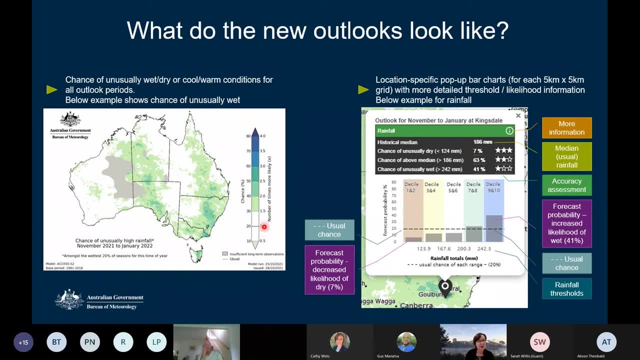 the wettest 20 percent of the seasons. usually that um your usual risk is 20 percent, and so where it's shaded here is showing where the odds are stacked to being stacked towards, to it being more um an elevated risk. so here these green areas. so where it says, say, for example, a 40 percent, 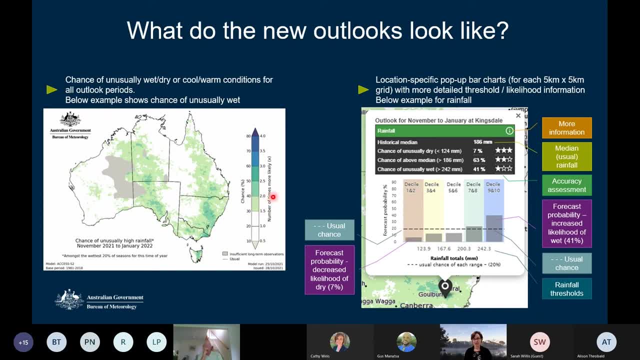 chance of it occurring. that's twice the usual risk, um, so it's an elevated chance. so you know your odds are now stacked towards you having, um, an increased chance of a of a weight, a high rainfall season, and then, if you were to click on the map or search for your location, you would come. 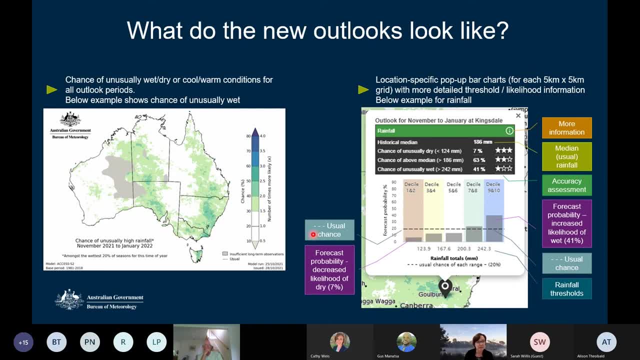 up with these bars. so again this bar. there's the usual chance, which is the 20 percent line. but now this bar shows more than this map, because this map here is just showing the unusually wet conditions. so that map is really only showing you this: decile 9 and 10. you know what's the chance you would decile 9, 10, these. 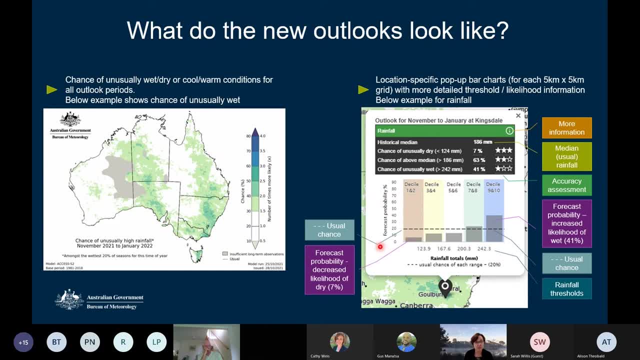 bars are showing you the whole um distribution. so it's showing you um that, um. so for this location, for example, the 20- 20 percent of driest seasons have rainfall less than 123 millimeters. the 20 percent of wettest seasons have rainfall greater. 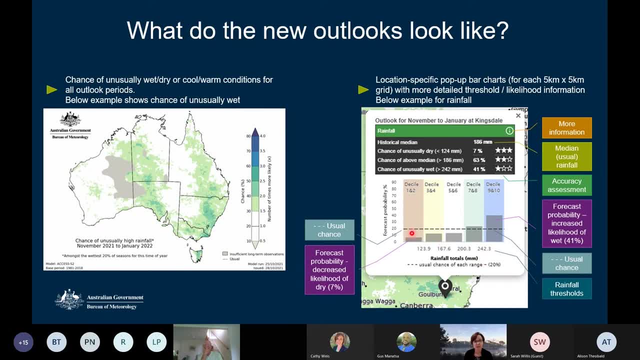 than 242 millimeters, and so usually there's a 20 percent chance of you having rainfall in any one of those categories. and then we run our 100 forecasts and say: well, what is the forecast indicating? what are those 100 forecasts saying? um that the rain, where the rainfall, will fall. 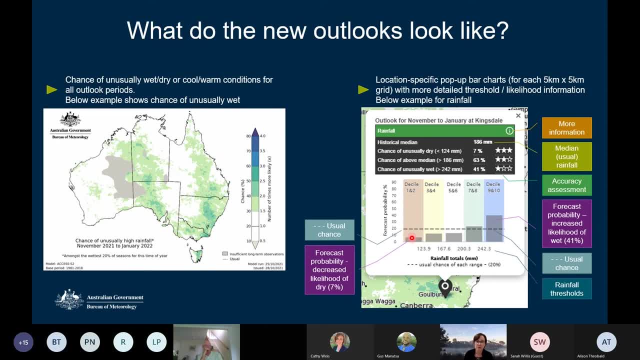 and you can see that's what these bars are showing. so it's showing that those 100 forecasts are showing that the rain is going to have the highest chance of you having rainfall in any one of those categories. so we can do the çam um. so 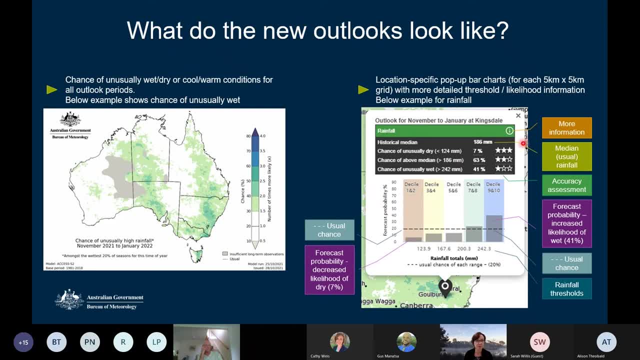 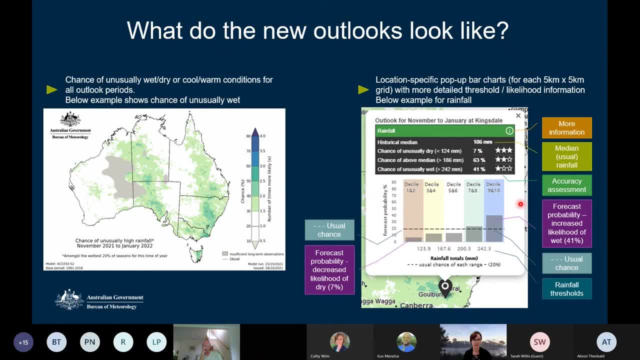 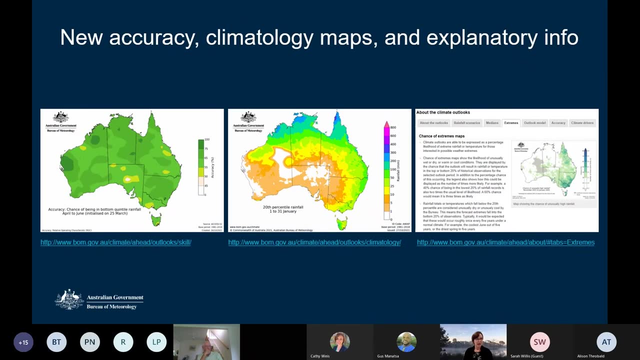 The chance of above median- that tells you- and the chance of unusually wet. Then the stars here indicate the accuracy. Three colored in stars mean good accuracy, whereas one colored in star means accuracy is probably quite poor. The same that you get with your probability of our median maps. 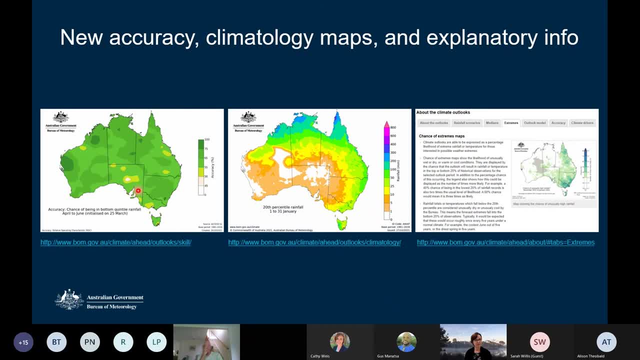 you can also click on the website to find out the accuracy. Those bars told you what say your threshold was for your wettest seasons or your driest seasons. But you can actually also have a look and see in a map what that means. 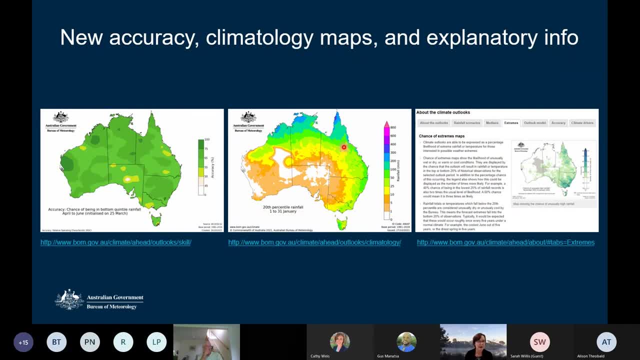 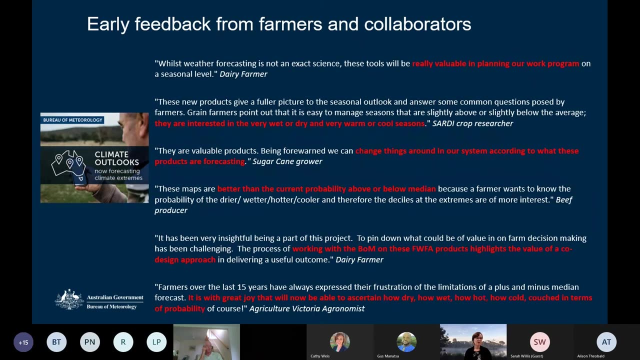 This is showing your 20th percentile rainfall. Rainfall less than these amounts would mean that you had a very dry season. Then there's information that explains more about these new products. We've had some early feedback from producers and from collaborators, Some of them I just put here. 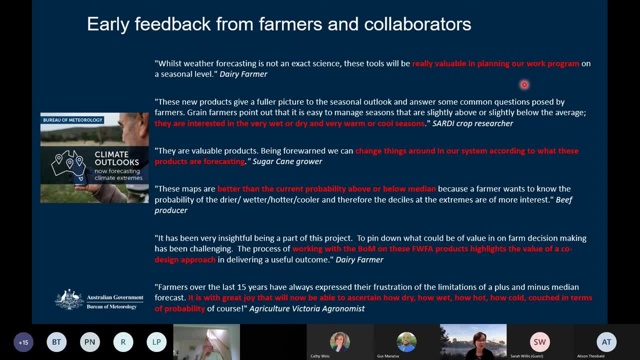 The tools are really valuable in planning our work program. A lot of the comments have come that managing a slightly above or below you can't do that Average season is easy, but really what we want to know is: are you going to have a very wet or very dry or very warm or cold season? 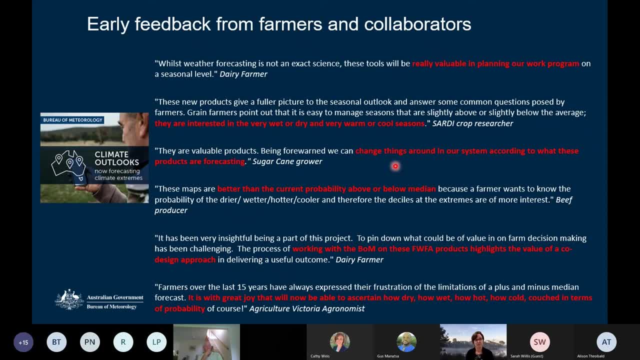 Being forewarned means that you can make decisions based on what the products are forecasting. This comment here about working with the Bureau on these products highlights the value of a co-design approach. That value means that, from Bureau perspective, we get insight into 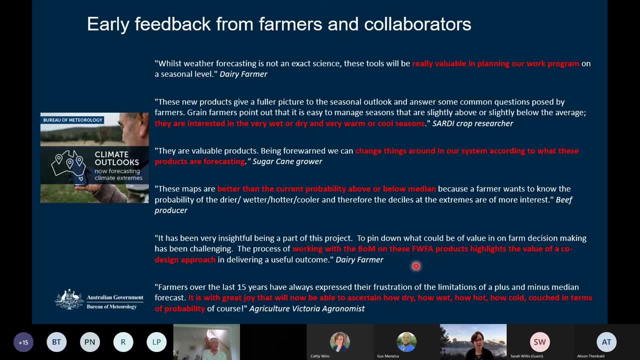 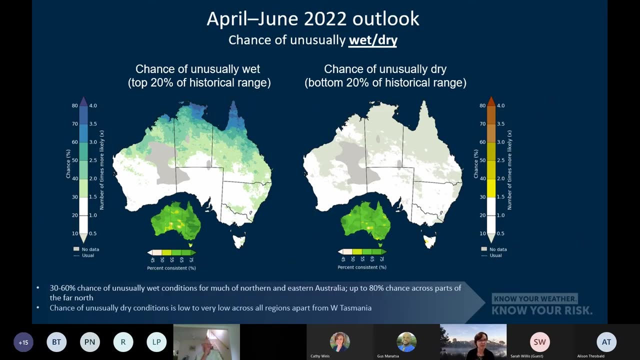 into the kinds of decisions that you make, the kinds of forecasts that you need, and also how we can actually better communicate those forecasts. Now I'm going to just show you what the current outlook is, but show it with these new extreme products. 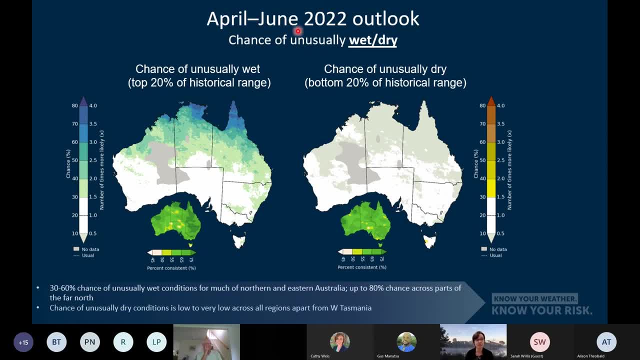 This is the April to June outlook for this year. This outlook is showing what is the chance of being unusually wet or dry. The one on the left is showing what is the chance of it being unusually wet, So what's the chance you're going to have a rainfall season that falls in. 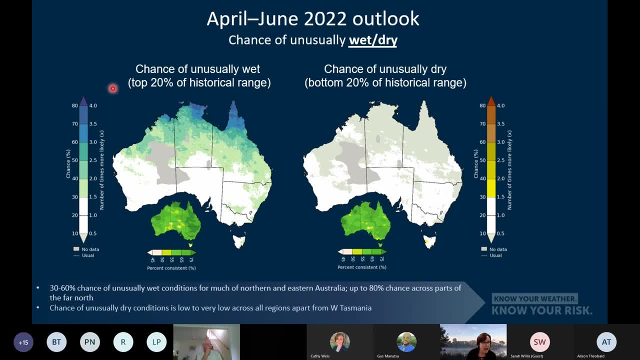 the top 20 percent of the historical range And the green light- green here, so for parts here of Eastern Australia- are showing, you know, 30 to 60 percent chance. I'm unusually wet And so a 30 to 60 percent chance means one and a half to three times. 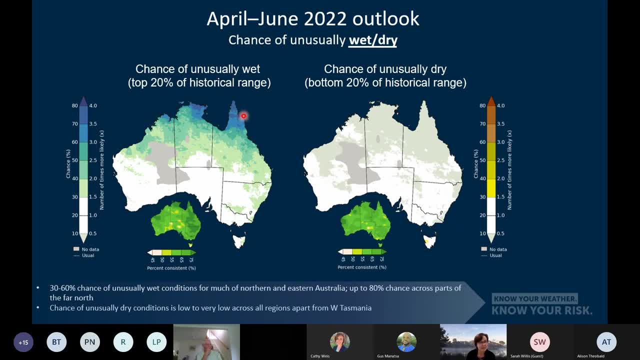 increased risk compared to what you normally would have, And some of these areas here in the top end in the far north. there's up to 80 percent chance, So the odds are stacked towards having a very wet season, If we look at this. 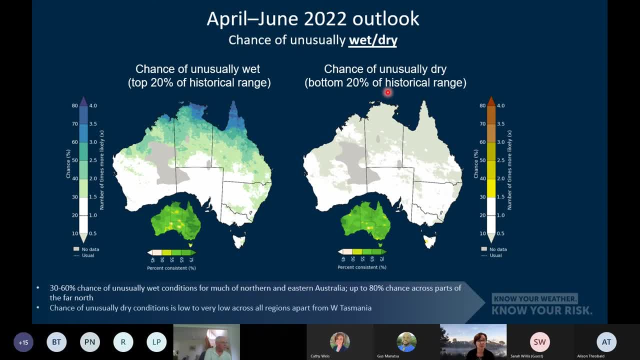 this is now the opposite. What's the chance of it being unusually dry? So what's the chance of it being in the bottom 20 percent of the historical range? And you can see that for most of the map it's this sort of like gray. 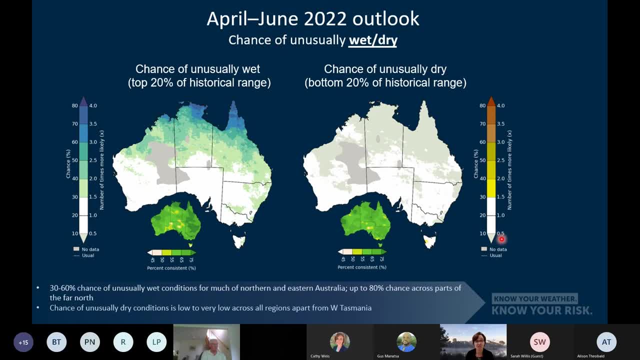 light gray color and that means strongly reduced chance. So there's a reduced chance that you're going to have a very dry season. On the other thing to note on these rainfall maps there's this funny shape, gray shape. That's a mask, just masking out areas where there's very few observations. 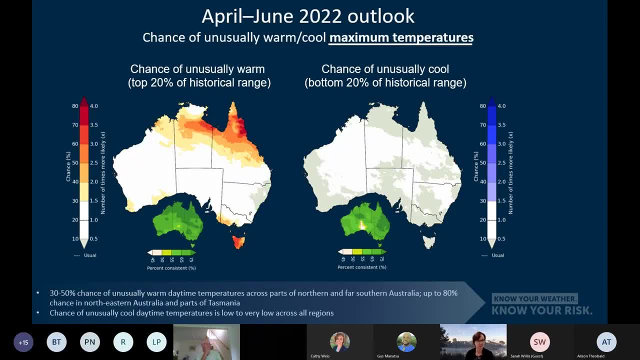 If we look at the outlook for April to June for maximum temperatures- so daytime temperatures, you can see that there's a strongly increased chance of having a very warm April to June In the top 20 percent over northern and eastern Australia and there's low chance of having unusually cold conditions. 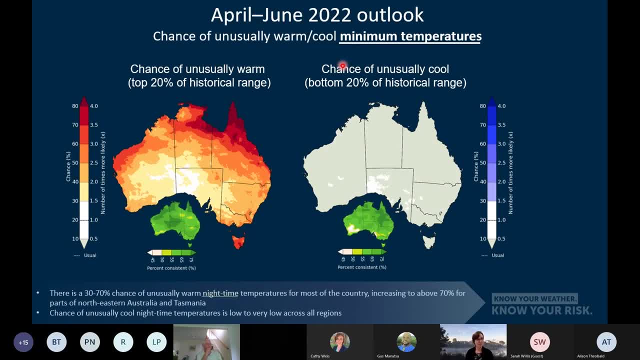 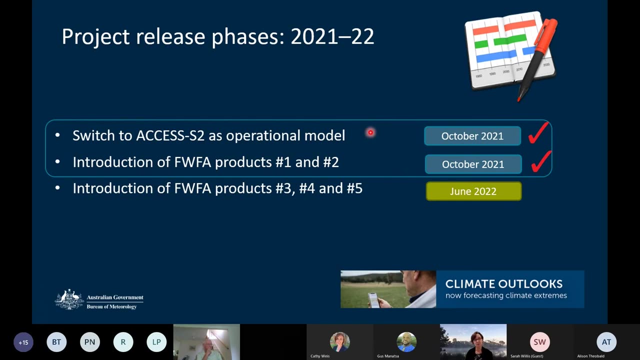 For minimum temperatures, so nighttime temperatures. most of Australia is showing an increased chance of having really warm nighttime temperatures. So what's next for the project? So we've switched to XSS2.. So when we switched to our new operational model, that's when we also introduced the new products that I've just shown you. 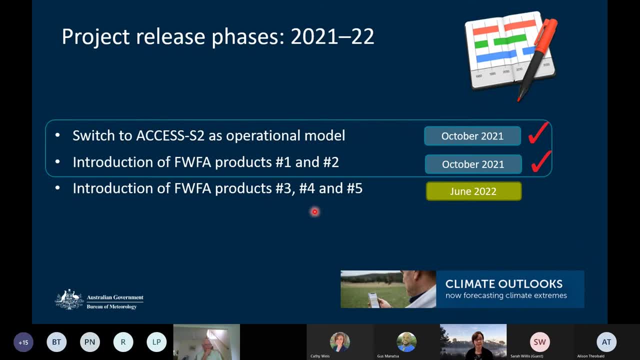 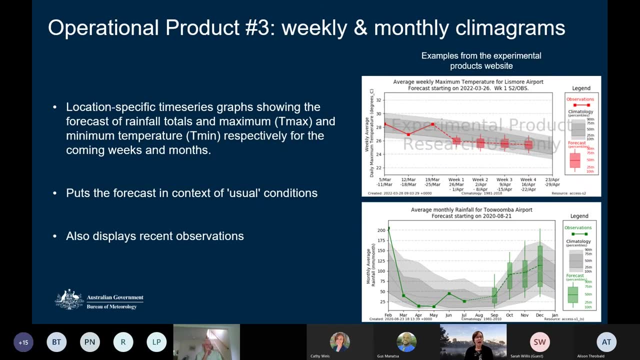 But then in June this year we're going to be releasing the next three products on the website. So I'll just show you a little bit now about what those products are. I'm showing you now these products as they look in our research website. 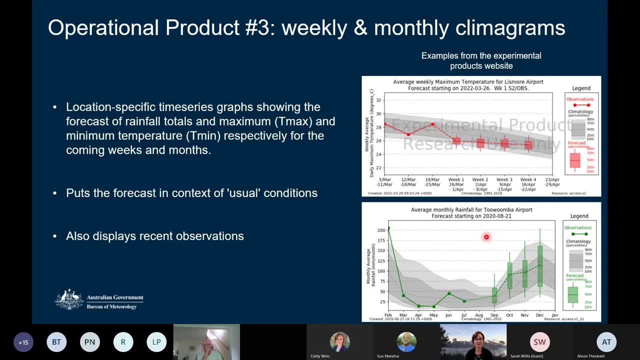 So not what they're going to look like when they actually appear on the Bureau's website. When they actually appear on the Bureau's website, they'll probably look a lot better. they'll have better text, Anyway. so this product is what we call our weekly and monthly climograms. 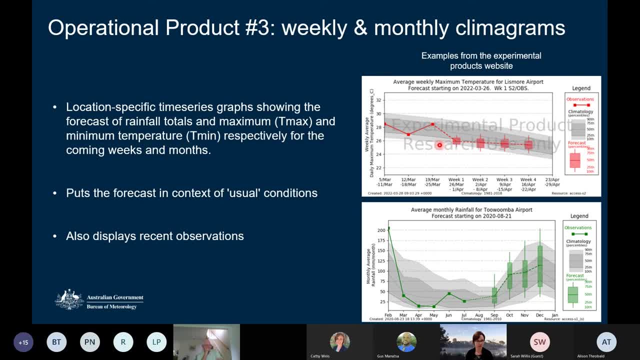 So it's a location-specific product for rainfall and temperature. At the top here I'm showing an example for the weekly product. So it's essentially a time series. So it shows past weeks. So the solid line here shows the so on. the y-axis here is your maximum temperature. 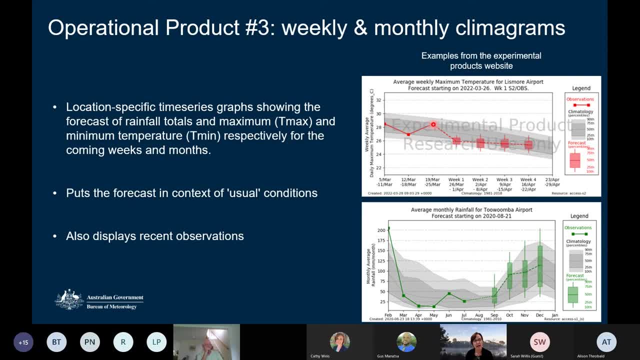 It shows the weekly maximum temperature for some past weeks, and then the dashed line with these boxes show the forecast. Now, what these boxes show is the range from those 100 forecasts that we ran, So you can see how certain or uncertain the forecast is. 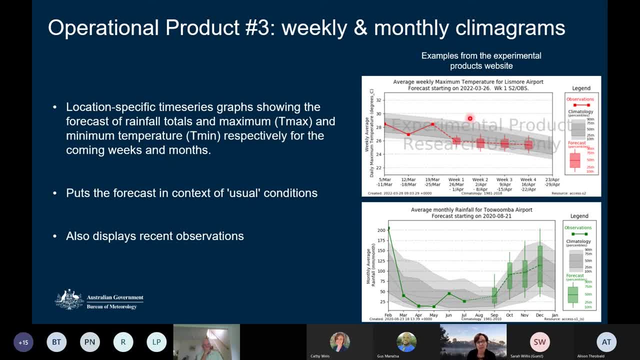 how wide is the spread? In the background, in gray, is actually the usual conditions for that time of year. So this middle gray line, if you'd see, here is the median, the usual median. So in this forecast here for the week one, 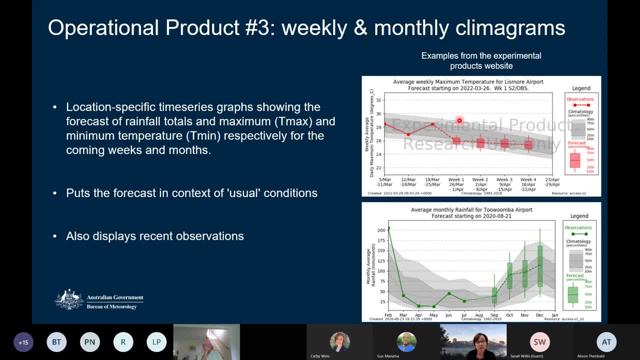 this box is lying quite low down compared to what's usually expected. So it's putting the forecast in the context of what's usually expected. So it's a CUDA forecast than you would normally have for that time of year. So that's just added information. 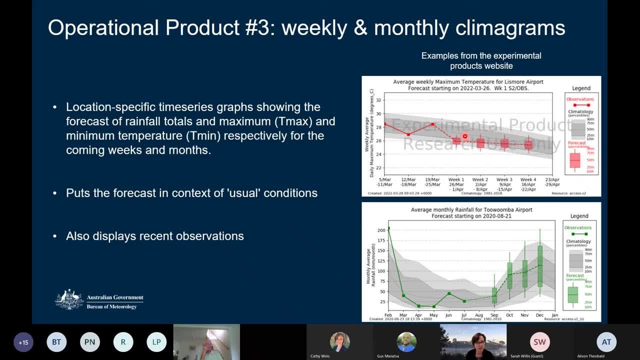 You don't have to compare it to past conditions, because you can actually just look and see what the actual temperature is that it's being forecast. Equally, there's also the monthly time series, So the solid line shows past months of observations. 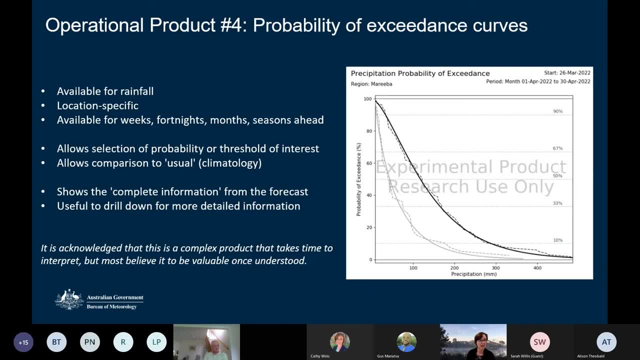 and then the bars show the forecast. Then this is another product which is available only for rainfall, and it's what we call our probability of exceedance curves. Again, it's a location-based product and it's probably the most complicated product. 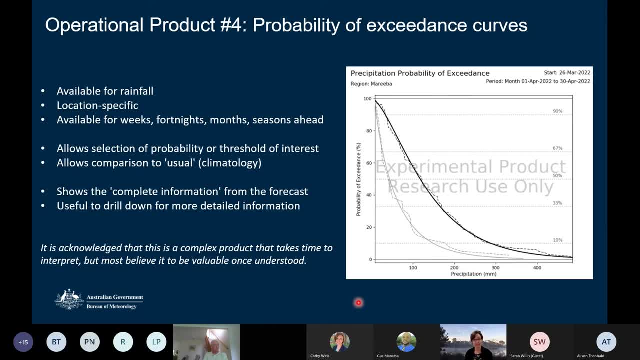 In some respects, we were quite surprised that it ended up getting selected, But I think that it's a complex product but it's quite valuable once it's understood how to use it. So really, what it's showing here is on the x-axis is rainfall. 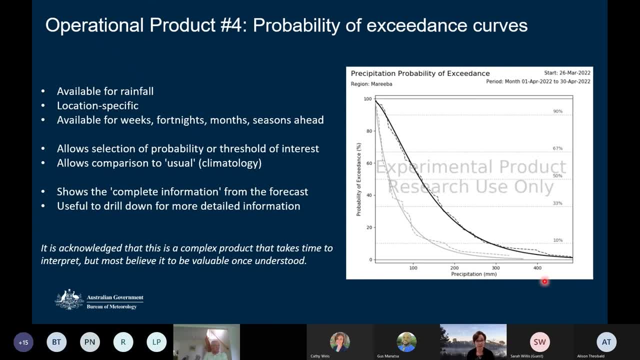 rainfall totals and this is available for weeks, fortnights, months and seasons. So this example here is for a forecast for the month of April coming up. So rainfall totals for the month of April. The black line: don't worry about the dashed lines. 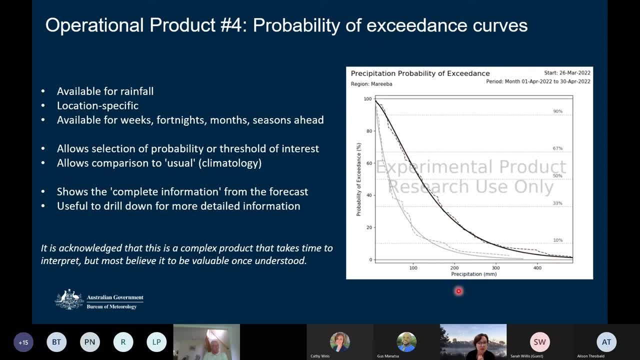 but the black line is the forecast, So you can pick a rainfall amount that you're interested in, say 200 milliliters of rain, and you go up and you then go across and you see it's got about a 25 percent chance. 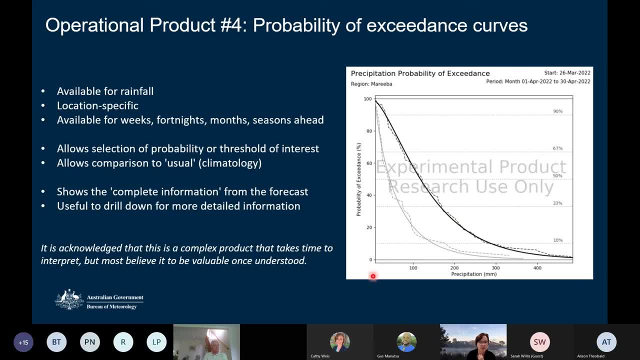 of getting 200 millimeters of rainfall, So you can select whatever threshold that you're interested in. The other use in this diagram is the light gray line, because the light gray line shows what usually happens for that time of year for that station. 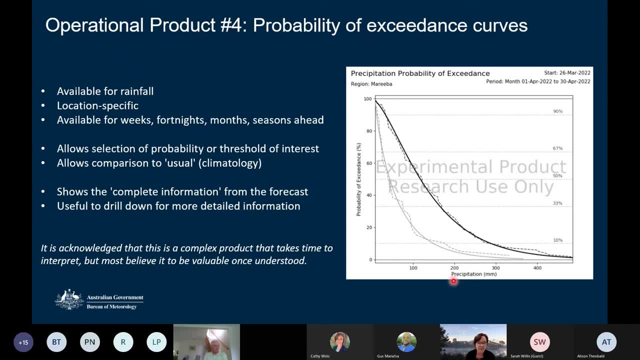 And so you can see if we look at the, say, 200 moles, usually there's only like a 5 percent chance of getting 200 moles. So the fact that this black line is above it is showing that it's a much. 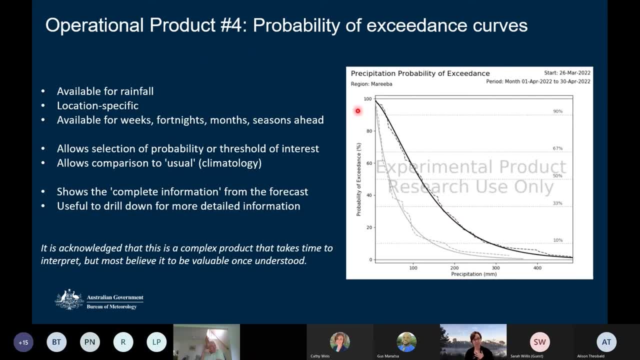 way to forecast. Another way to look at it is that these curves all slope from the top left down to the bottom right because essentially you know you've got a greater chance of having smaller rain full amounts And then, as you get to higher rainfall amounts. 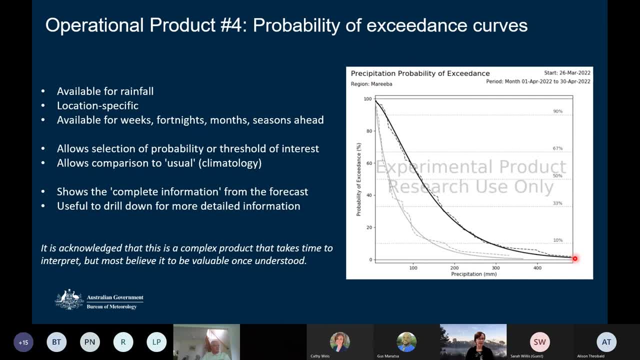 the chance of you having them decreases. So essentially this product allows you to sort of select whatever rainfall amounts you're interested in and delve more deeply. So some users are not going to be interested in this kind of complex information, but there has definitely been interest from other users. 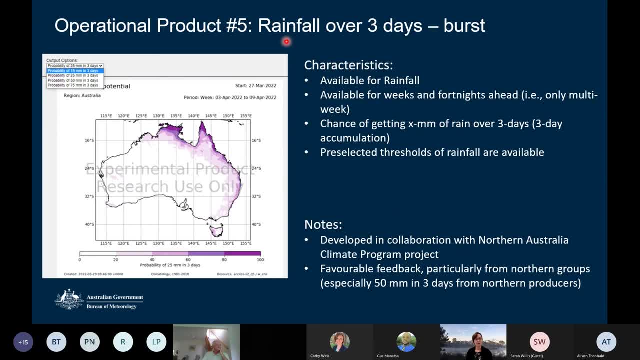 And then the last product is what we've called the rainfall burst And basically it's looking at the rainfall that might happen on over three consecutive days, So trying to get at you know might there be, instead of looking at like over a whole week or a whole fortnight where you don't. 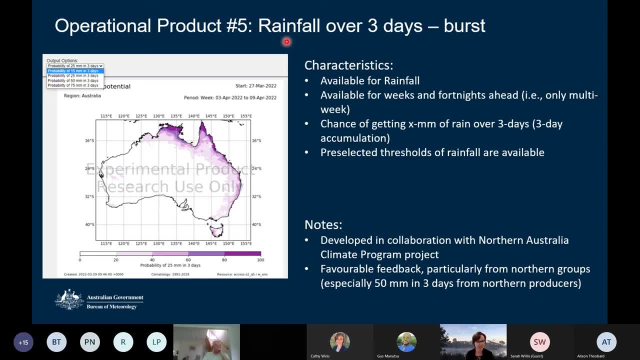 know if the rain's fallen as drizzle over the whole week or whole fortnight. it's looking at more. you know what is the chance I'm going to actually have a burst of rainfall, And so what it is is we've got different thresholds. 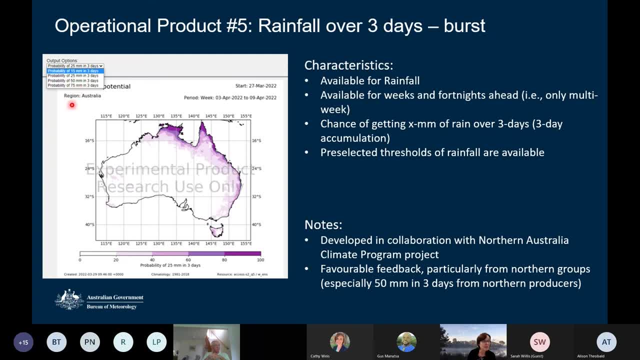 So you can select a threshold, So say 50 millimetres of rainfall in three days or 75 millimetres of rainfall in three days, And then it tells you the chance of actually getting that, And this is available only for the weeks and fortnights ahead. 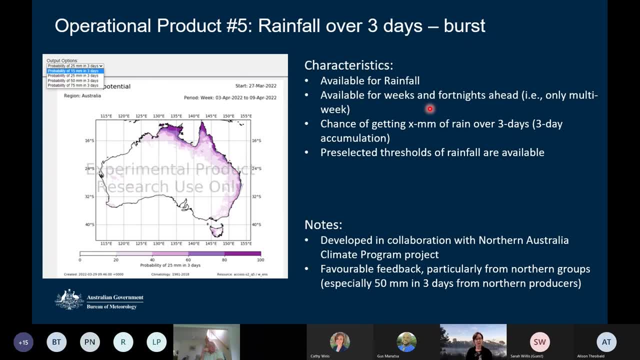 And this product in particular was very useful, had very favourable feedback from our northern groups, particularly the livestock industry, And you know, one of the things they're really interested in is something like 50 moles in three days. So essentially that is our portfolio of five operational products. 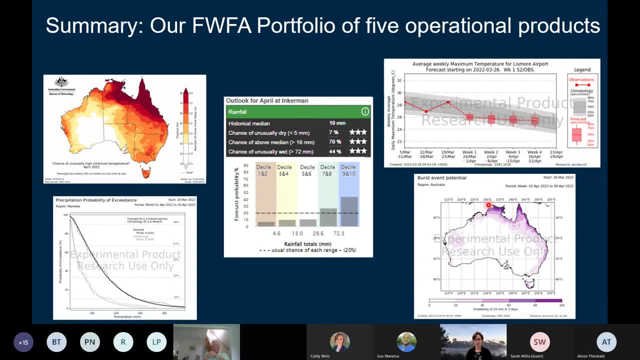 Two are already operational and then these remaining three are going to become operational and visible on the Bureau's website in June And, as I said earlier, because we have several different agriculture sectors, as you can see, they're not tailored products. They don't have sort of tailored indices, growing degree days or whatever it might be. 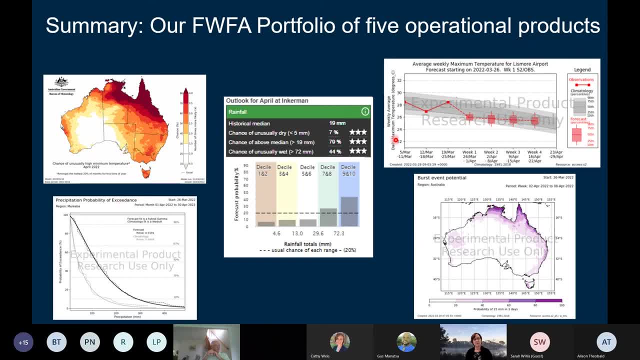 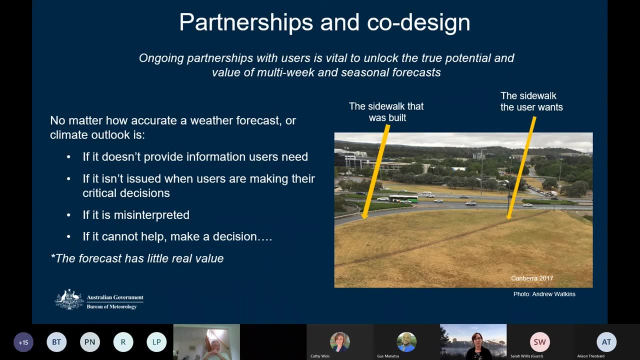 But that also means that these products are probably going to be useful for a whole range of sectors, not only agriculture, and also different use cases. So, finally, the last point that I want to leave with you is: I think that really the value of this project has been in the co-design and the engagement. 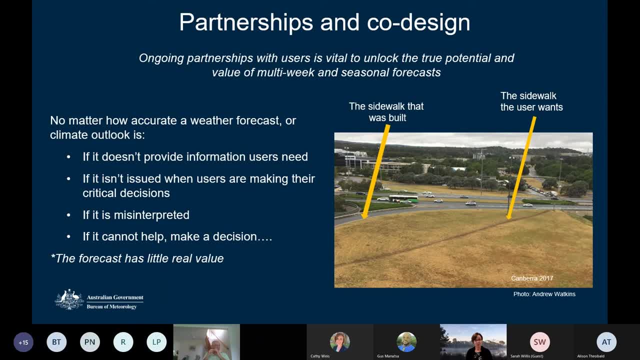 And I think that we really need to do more of this, because it really does help with with communication, with actually influencing the final utility and understandability of the products that we produce, And I've just got this little diagram here. So, basically, no matter how accurate a weather forecast or climate outlook is, 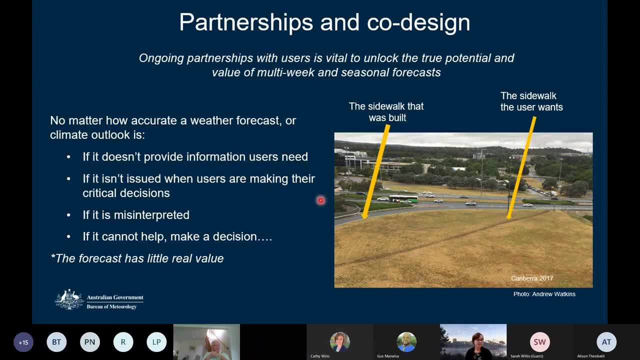 if it doesn't actually provide the information that you need, if it's not issued when you're making your critical decisions, if it's misinterpreted- and that often happens with probabilistic forecasts which are challenging to interpret- And if it can't help you make a decision, then it doesn't actually have real value. 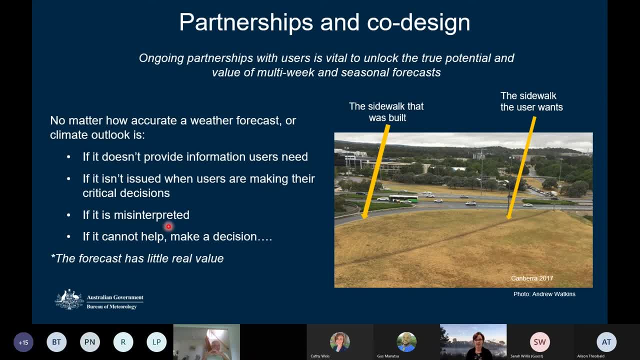 So that's why we really do need to have partnerships to actually kind of unlock the value in these seasonal forecasts. I really like this picture here. It shows: you know, this is the sidewalk that was built, but clearly this is the sidewalk that the user wants. 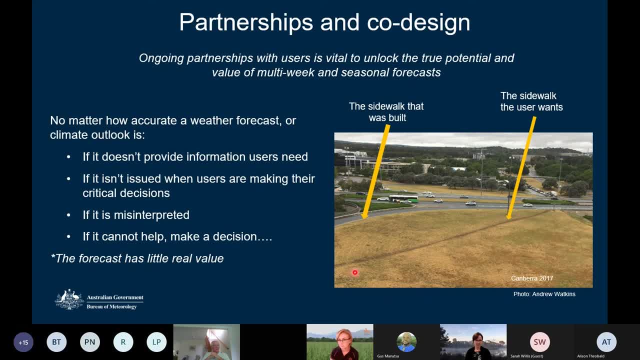 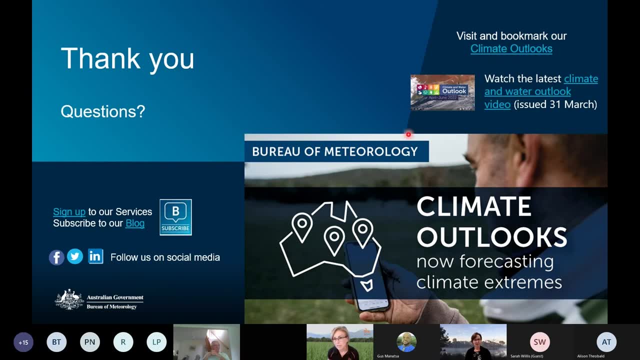 So the real value of engagement. So that's, that's it from me. Cathy, I'm happy to take any questions. So I don't know if, hopefully, you're all aware that we have, you know, climate and water outlook videos. So the latest video was issued on the at the end of last month. 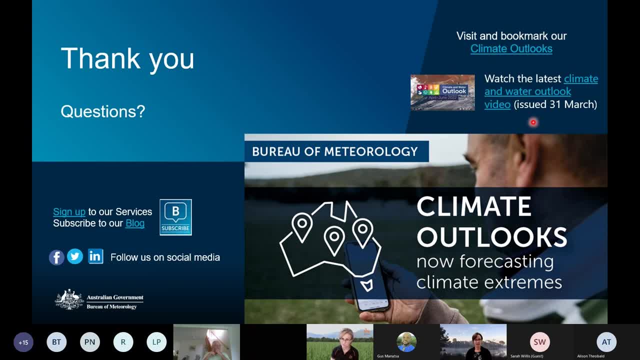 And that will take you through more of the forecast for the upcoming season. And yet those maps that I showed you all available on our climate outlooks website. Thanks, Thank you, Debbie. Look, I have reached out to people via chat. Please don't be shy if you have questions for Debbie. 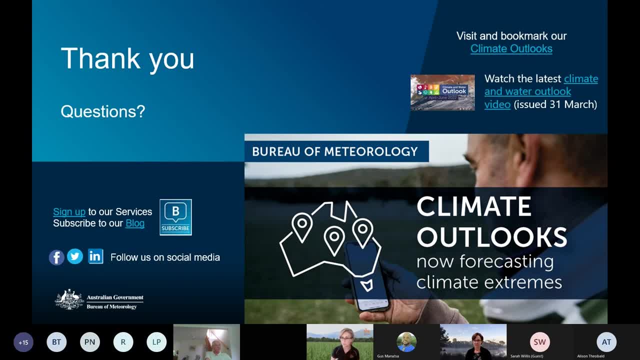 Please either raise your hand using the chat or, you know, feel free to type those questions in. Debbie, I have also shared the link via the chat to the video so that people have easy access to that. I guess, if I kick off with a question, 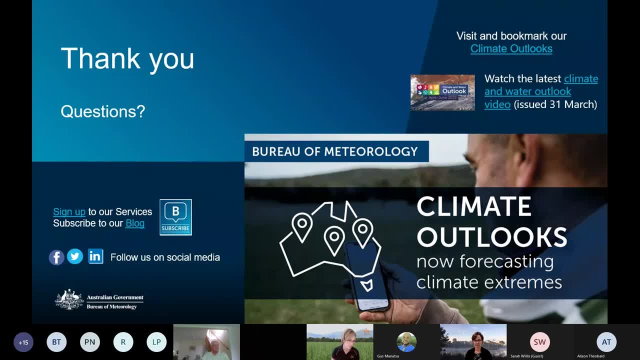 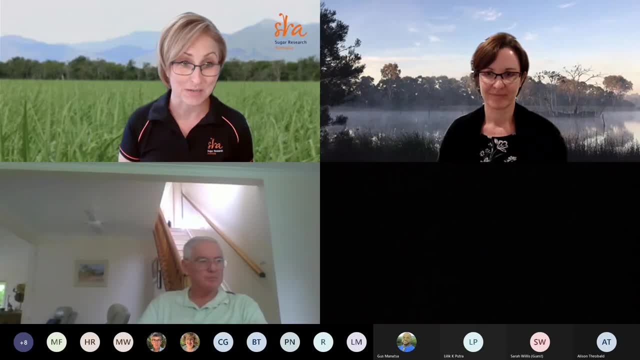 Okay, So I'm going to take a quick question while we're waiting to see if any others come through from our guests on the call. We obviously have recently seen some extreme weather in southeast Queensland and northern New South Wales. I'm interested in whether you've received further feedback about the usefulness of the tools since that time. 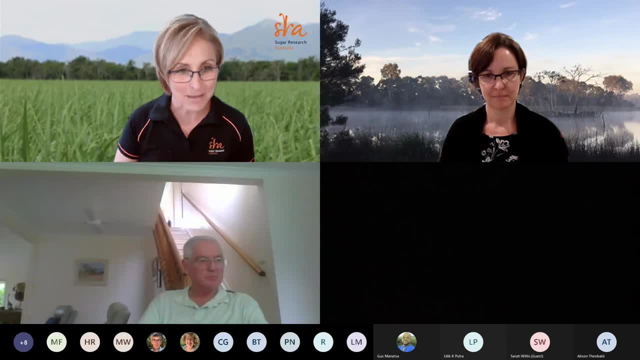 Certainly in the slides you shared some of the feedback from some of those users. I'm interested in whether you've received further feedback about the usefulness of the tools since that time. Certainly in the slides you shared some of the feedback from some of those users. 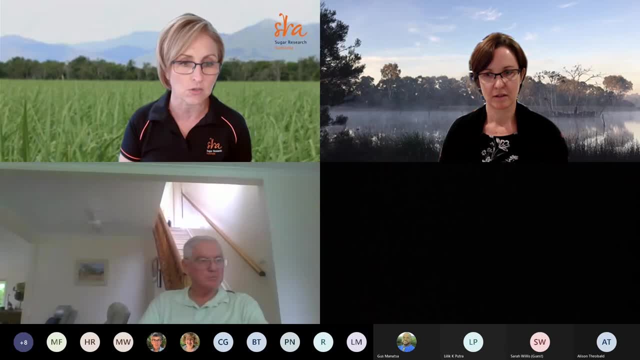 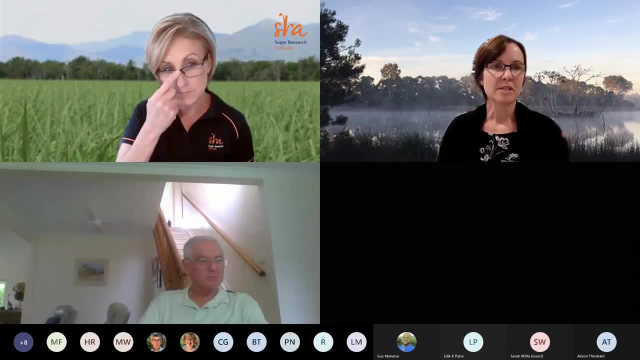 But has there been anything specifically in the context of the recent weather events? But has there been anything specifically in the context of the recent weather events? But has there been anything specifically in the context of the recent weather events? Yes, I would say that the feedback has mainly been on the forecast for the months and seasons ahead. in terms of that, 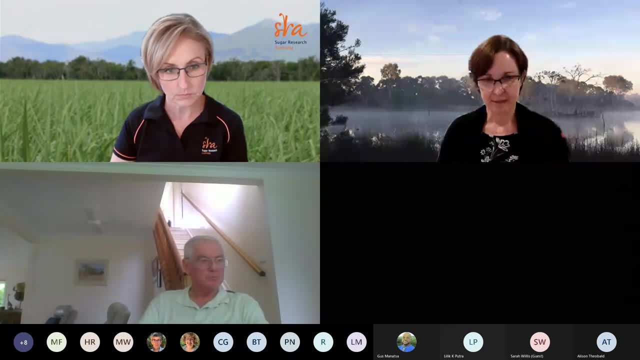 Yes, I would say that the feedback has mainly been on the forecast for the months and seasons ahead. in terms of that, Yes, I would say that the feedback has mainly been on the forecast for the months and seasons ahead. in terms of that, the forecast for the months and seasons ahead. in terms of that, so, quite consistently, our forecasts. 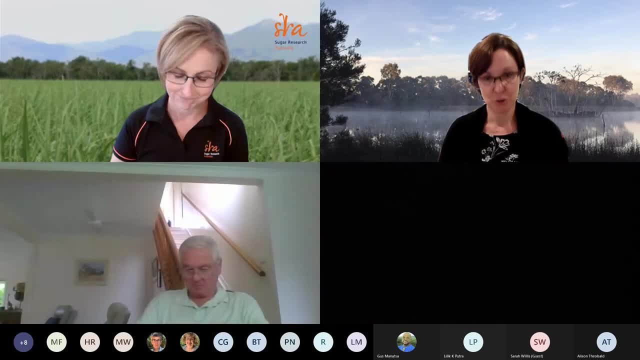 have actually been indicating wetter, much wetter than average months and seasons, over the last last few months and obviously that's eventuated over large areas and that's that's pretty much due to the fact that we've had this La Nina condition and again, I think it's. it's the 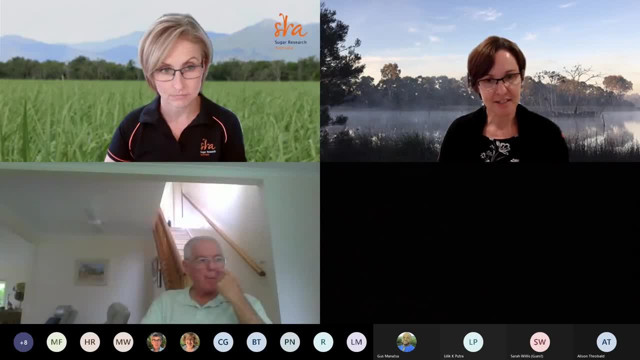 feedback has been about, you know, the insight into- not just you know- probability of above median. well, is it going to be just a little bit above median or is it going to be a lot above the median? and so a lot of the feedback has been on, you know, having having more insight into 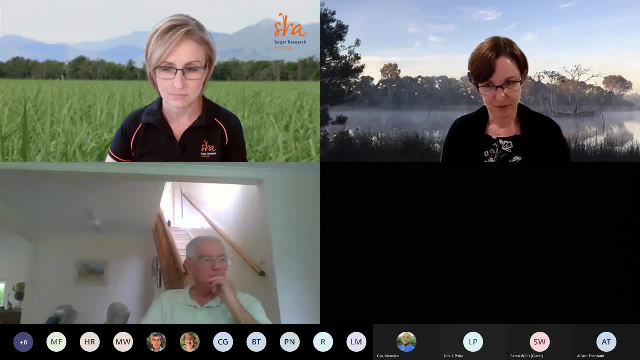 into what it might mean and how, how the odds might be shifted. look, that's certainly um some of the feedback I've heard from a user. um, and without stealing the thunder of um Friday's session, um, you know there will be a little bit of a salient lesson there in terms of, you know, 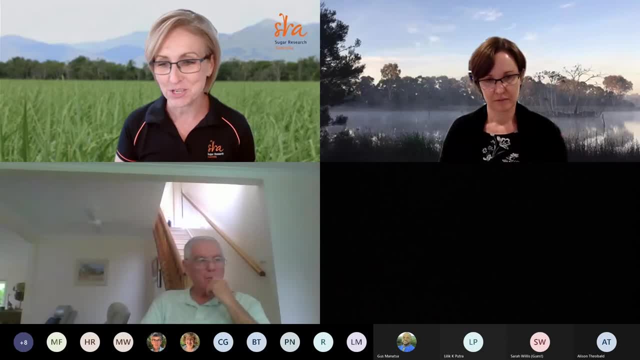 we were warned um and you know um. you know how um the tools may be able to influence or support decision making, um you know, within the the agricultural setting um. I see that we've got a question come through, Debbie um, from a person on the call um it's asking: 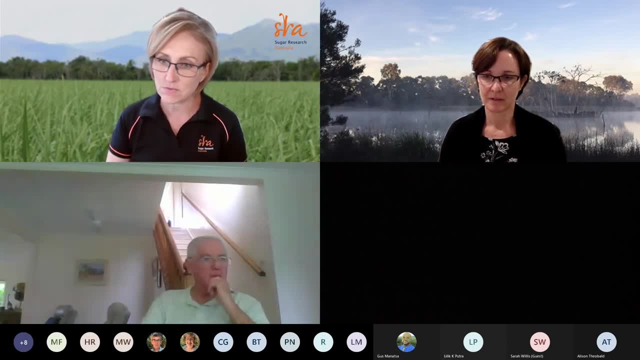 or indicating that there used to be a tool for predicting the date of the northern wet season. is the three-day burst tool a replacement for that? no, it's not a replacement, it's an addition. so there's still that um so um. what Michael's talking about is there's a forecast for. 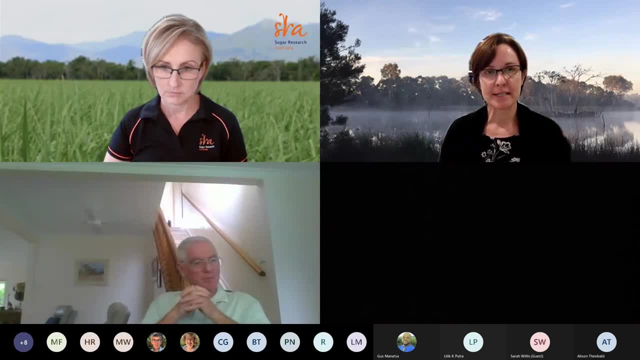 the onset of the northern wet season, and that's basically saying: um after you know when, after September, might we have had an accumulation of 50 millimeters of rainfall? and and that was sort of coming up um, that was devised in conjunction mainly with livestock users. um, as in that, that 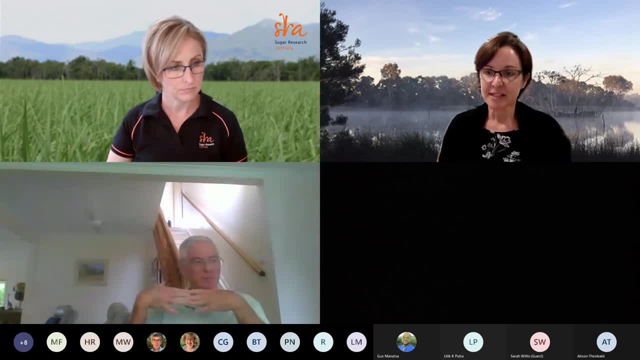 would. that's really when the pasture starts being available, and so that's saying you know that actual product is is saying are we gonna expect the- um, the wet season to happen earlier or later than we normally would so say you know, so say normally you would expect the wet season to start on the 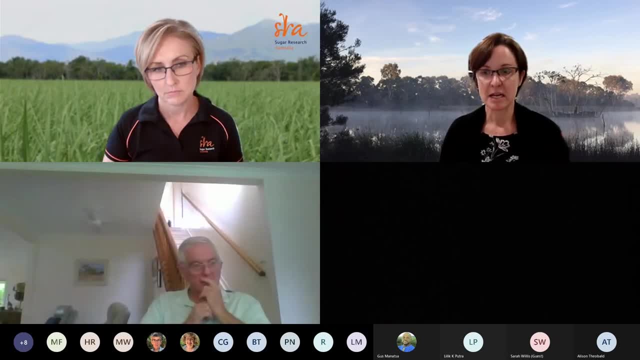 first of February, um, you know, are you expecting it earlier, later, so so that's still available. the first tool is more of a what might happen in coming weeks, um, and, and so it's, it's um. so it's saying, you know, well, in the next few and and it's, and it's um available the whole year. round, so that um start of the wet season is really just when might the weight season start? this first product is looking at um three-day rainfall accumulations throughout the whole year, so it equally might be useful for southern producers in in winter. you know an indication of, of bursts of. 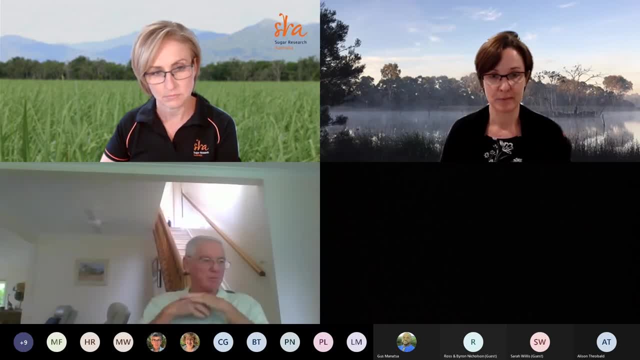 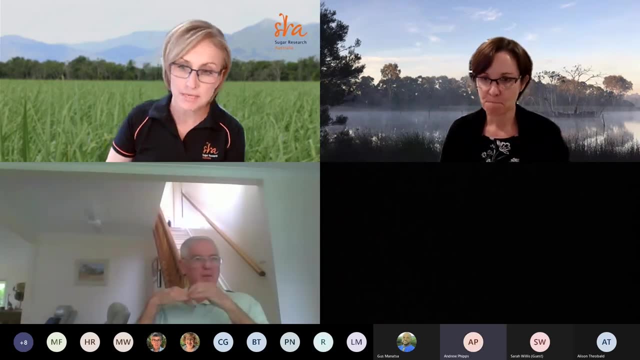 rainfall um and of different amounts, so not only that 50 millimeters of rainfall, so so it's an additional tool. thanks, Debbie. look some feedback. uh, also from me saying thanks for a great presentation. he does ask whether there's a contact for support um as end users start using the tools. 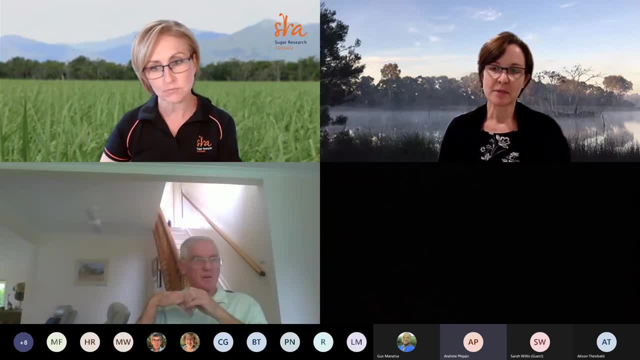 in their businesses? yeah, that's a really great question, so I would say that the best contact um is, so the bureau has um got um set to um groups there. so there's, we have an agriculture program um and I'll um maybe look and get the actual um website link and put it in the chat in a moment and so, um, the best is actually. 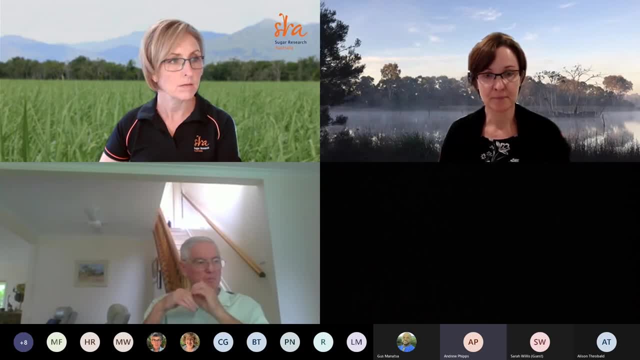 to make contact with our ag program um staff and then they will be able to either help you or be able to channel you to the right um people who might be able to to help you. uh, just solve one of those tips that you shared, Debbie, and when we caught up recently. 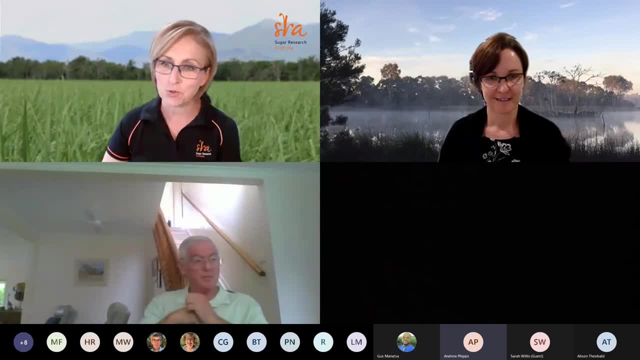 um, you pointed it out to me and I know you pointed it out again today, but as someone who was, um, I guess, noodling around in the tool, um that search, um magnifying glass to actually really be able to hone in on your location is invaluable, um, and not immediately. 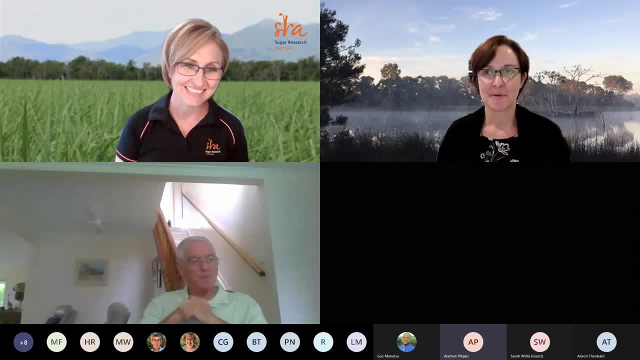 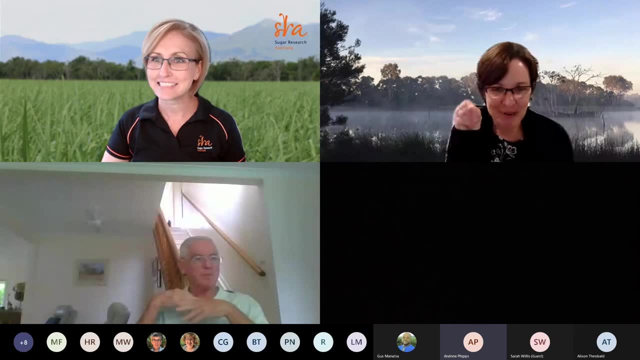 obvious to people, right? yeah, exactly, um, yeah, it really shouldn't be so hidden, um, but yeah, so um, you don't have to like, oh my gosh, where's my location? can I click on it again, you know? enter in your location's name and select it from the list. yeah, and look, uh, in, um, the reality is it's probably not. 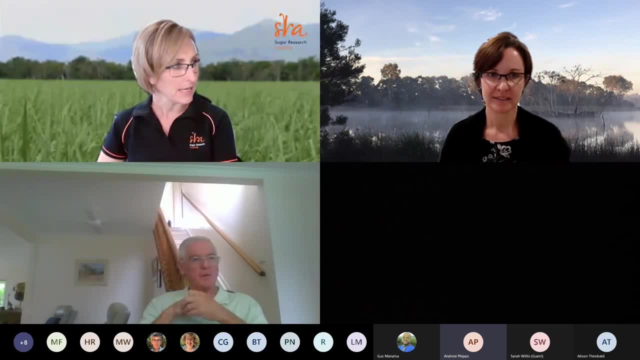 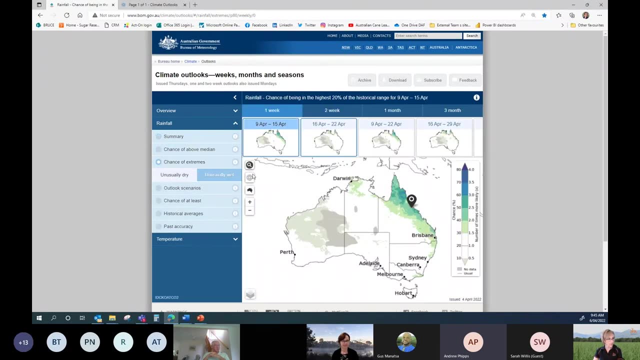 that hidden. I've just um jumped into to screen share um. hopefully people can see that I'm in that um extremes tool, um and um, I guess um for the benefit of others. on the call um, I had been sort of uh, trying to click in and and find the location of a particular 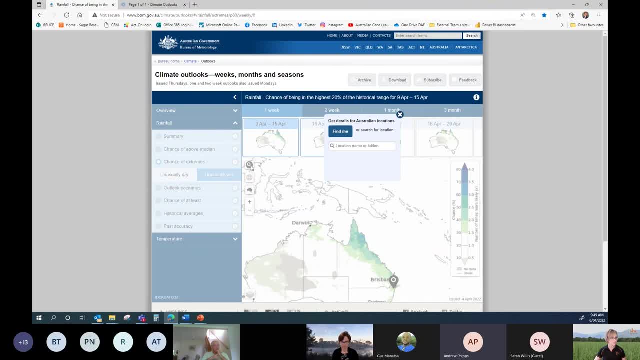 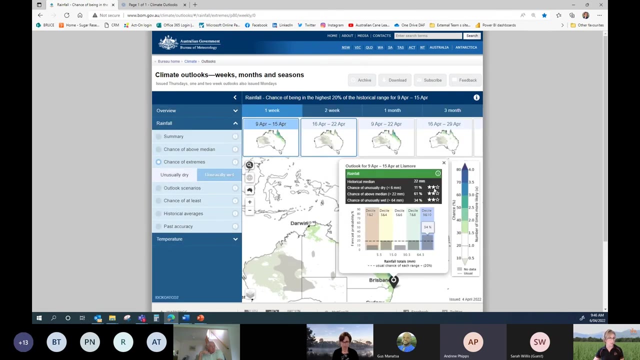 um place that I was looking for. but by clicking on that magnifying glass over here, it really is as simple as um typing in our location, um without the typos, and um um going in to see what's going on, um through there and um jumping ahead to sort of see what. 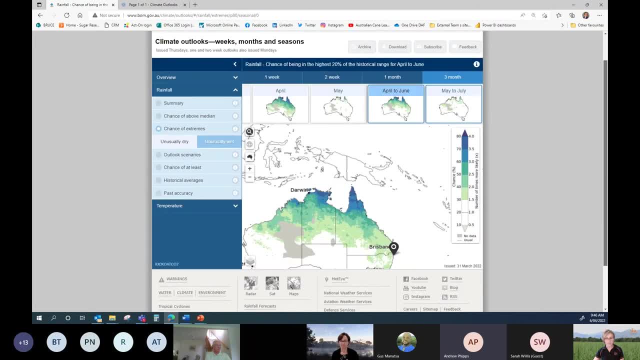 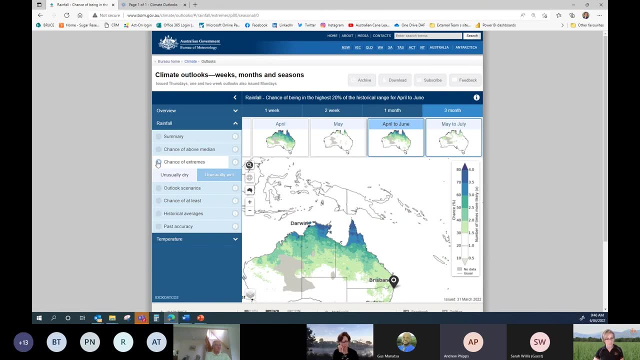 um, things are looking like over the next few months or the time frame that you're looking for. so, um, certainly um. you know I'm no weather guru, but um, it was fairly simple to to try and navigate um through that um, but certainly that little magnifying glass tool, um. 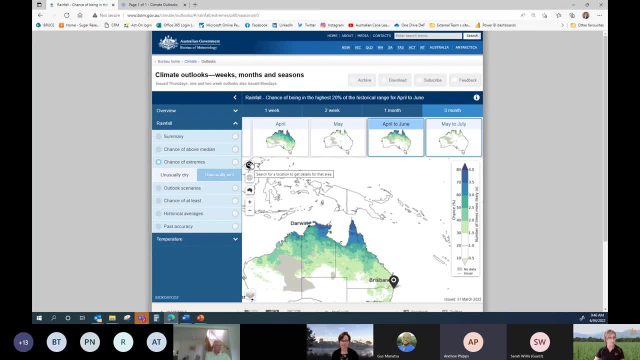 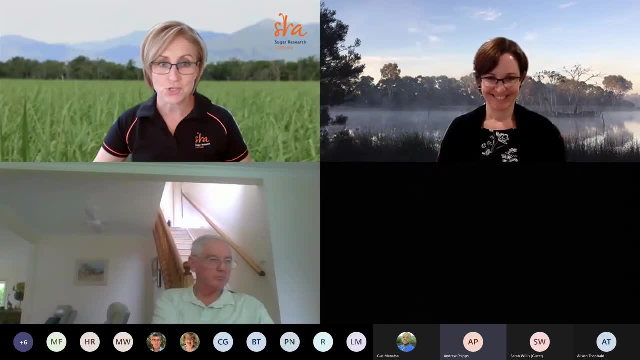 was a fantastic lesson, um, and I'm sure will help other users. sorry, I just stopped sharing. did you want me to share that again? no, no, that's good. I've seen that Christine's asked um. you know she's asked: what specific features do you need in order to make a? 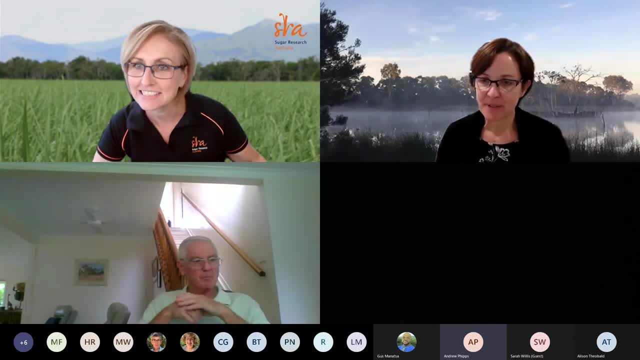 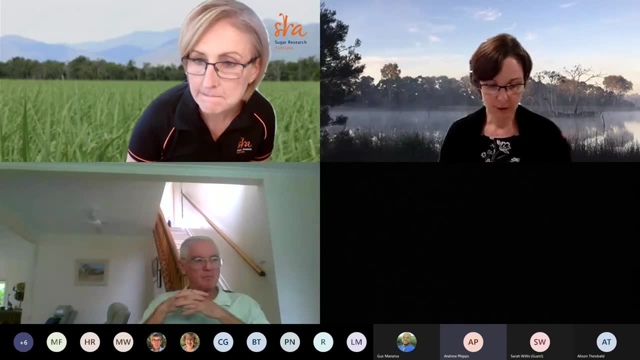 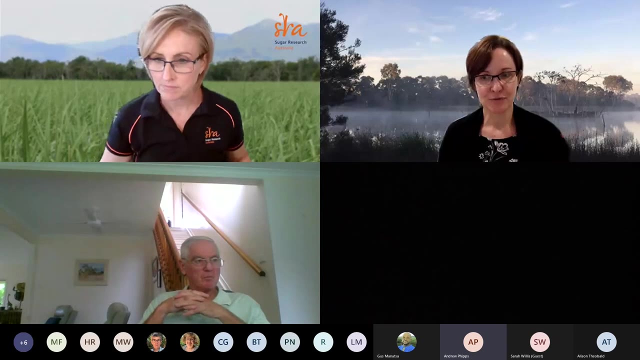 about, um, any details of the birdship cropping group's extension and work that they're doing with their growers, um, so, um, a couple of things. um, birdship cropping group have a website called climate kelpy um, which, which actually has quite a lot of useful blogs. so i've just done a blog. 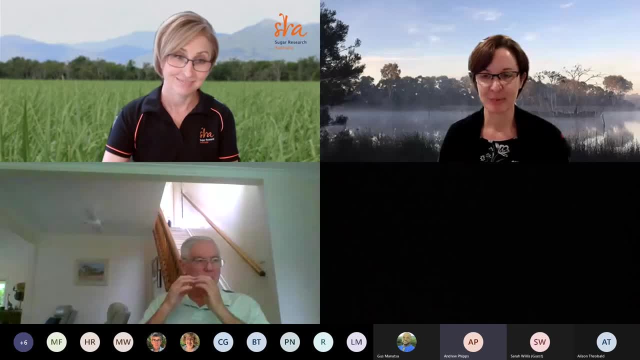 there about the move from access s1 to access s2, for example, and i think, kathy, you've done one recently or um, so so that's quite a useful um resource. um. they also, as i mentioned in the presentation, they actually run our monthly um community of practice sessions. um. so, if you are, 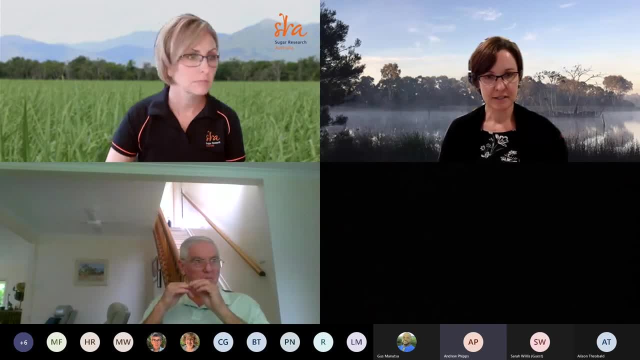 interested um, maybe i'll give kathy the details and um and you can be put on their mailing list so that you get um information about the um community practice sessions. they don't all um have, so each session is an hour long once a month and they're usually two or three presentations- they're not all on. 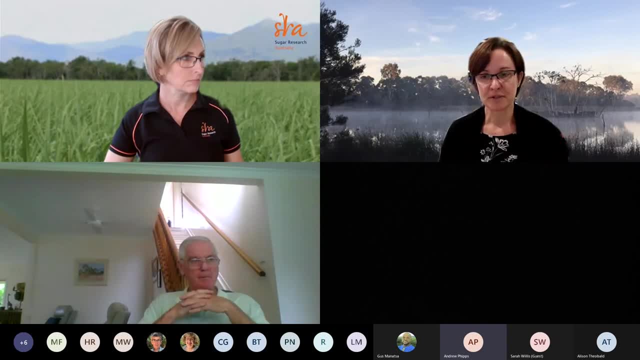 forewarned is farmed um. they're often on different um topics of interest to agriculture, um, so so it's a really nice um session i'll just share. i've got the climate kelpy um site um, oh, i'm not sure if that. yeah, it looks like it's going in as a link. it just says the words climate kelpy, but it does. 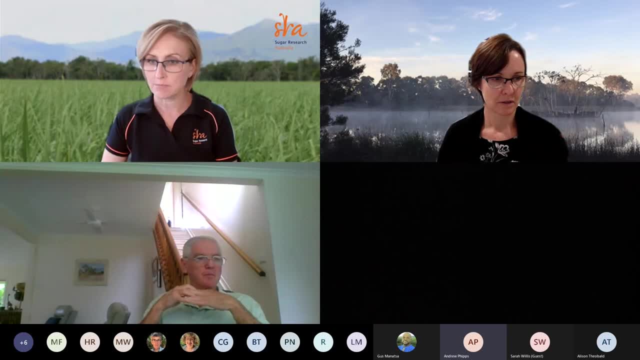 say, a lot of um weather and climate related information um on that site um, but yeah, certainly they've published some um some content in recent times uh relating to forewarned is is forearmed and to, i think, a number of the um different um agricultural groups who've been involved. 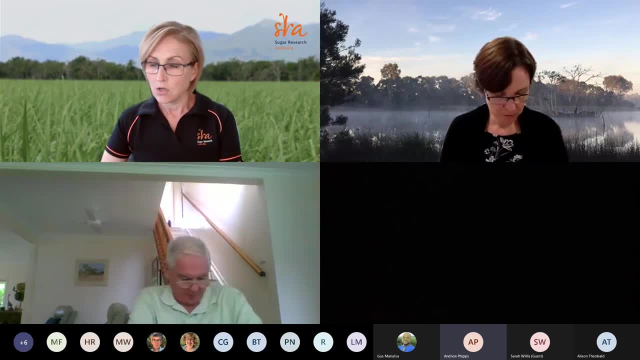 in that process. along the way, i'll put in information about the virtual cropping group sessions. now, uh, questions um from those on the line, um in your hands, about whether you have um anything else um in the meantime, debbie? um. another one from me: um, obviously, with climate change, we are starting. 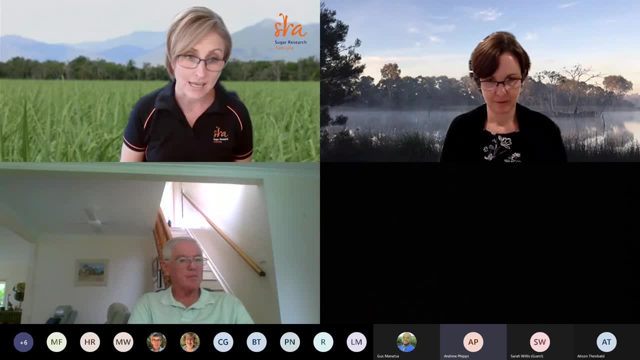 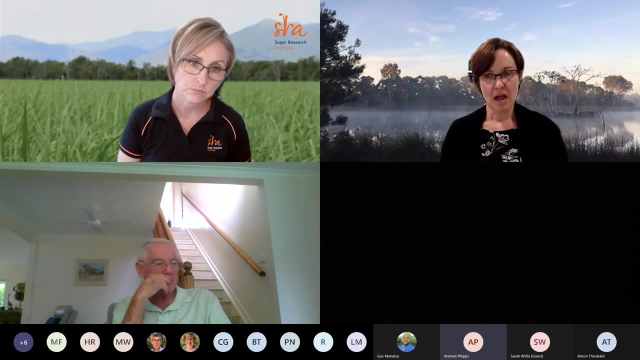 i guess, to experience some more frequent um extreme weather events. how critical do you see tools such as these that are being developed through? forewarned is forearmed in um in helping our agricultural sector. um very important so, i guess. i guess in the past, seasonal forecasts used to be constructed. 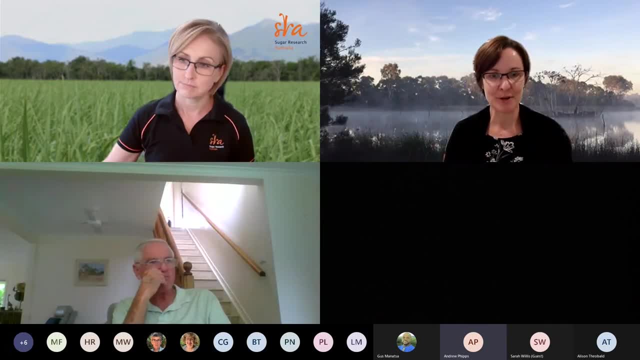 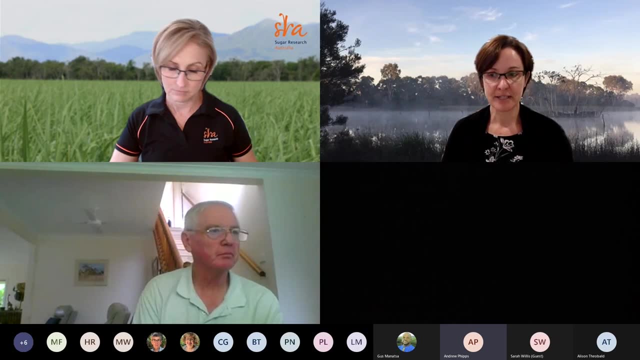 in a statistical way, which is kind of why i sort of started the presentation talking about the fact that these are models that are actually simulating what's going on. in the past, um, seasonal forecasts used to be created, um using statistics, and so what that meant is: you would look, say at, 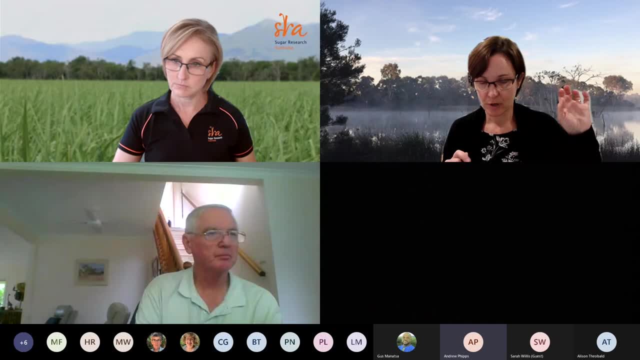 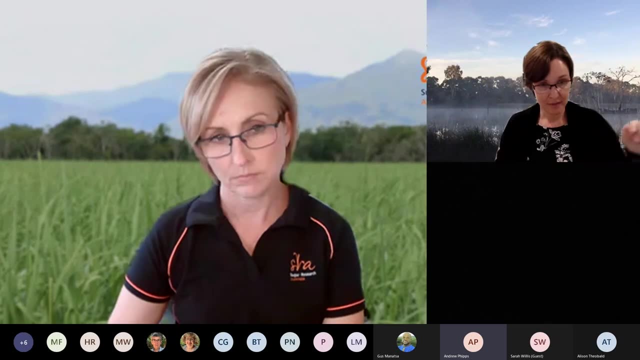 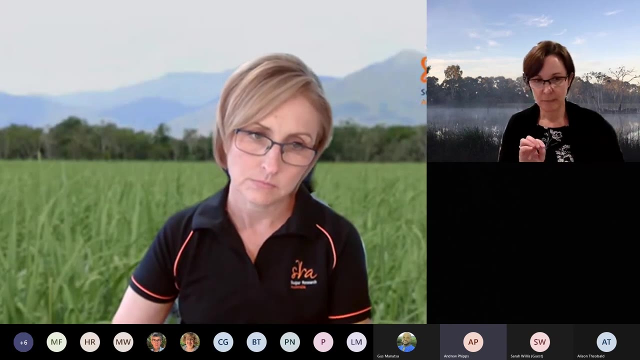 rainfall over australia and you would look at um sea surface temperatures in the pacific, so indicators of on year, and you would say: what's the relationship? um, and then you would apply that relationship going forwards. but so that relationship is um devised from looking at, you know, what's gone on in the past and so it doesn't actually um. so what we found is when statistical 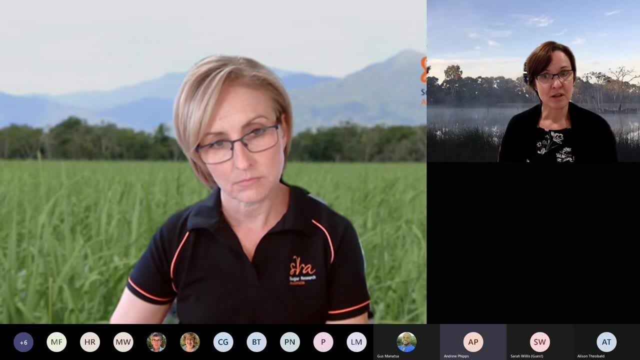 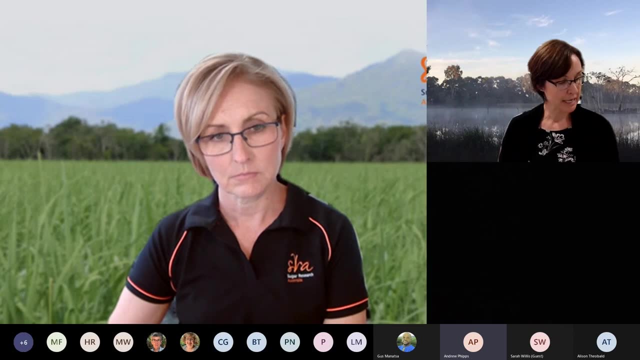 forecasts um started, you know, um not taking into account that the climate was changing, um, and so the one good thing about the dynamical models is that they can forecast conditions that we haven't seen before. um, they also do take into account, um, to some extent, that the climate is changing, because 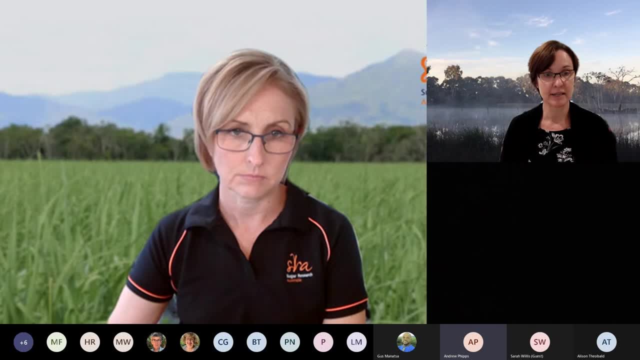 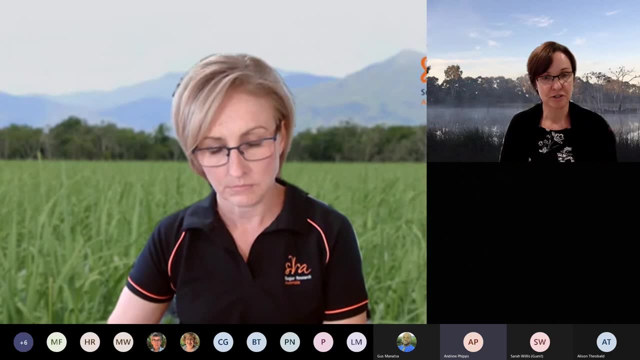 you. you can prescribe the amount of carbon dioxide and gases in the atmosphere in these models and they also obviously start. the forecast, as i said, is starting with the, the current condition, so it knows how hot the pacific is, ocean is, um, so that. so they having these forecasts are definitely a. 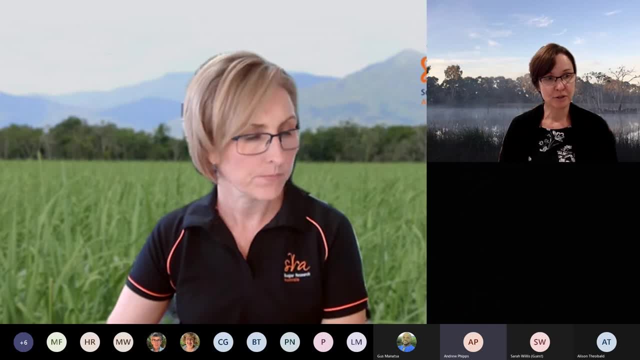 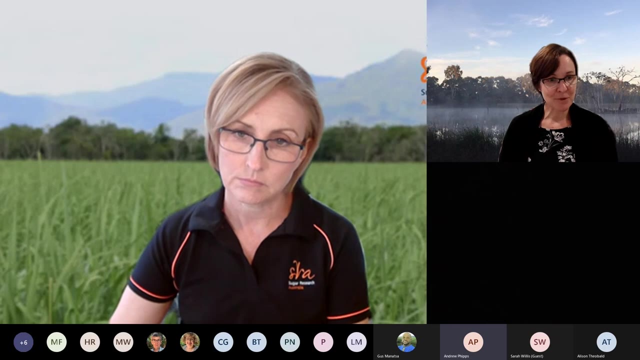 step in the right direction to um, helping with that um, and if you know, in terms of, like the northern regions of australia, the indications are for climate change, that um, you know there's an increase in wet season rainfall. so i think you know, just trying to increase the number of tools in in our 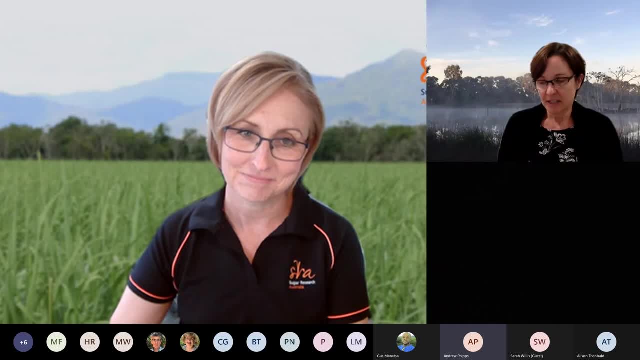 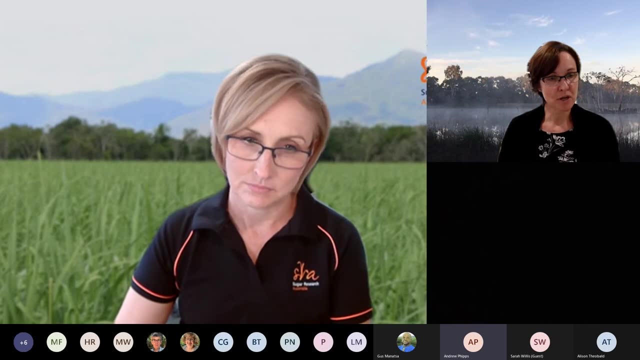 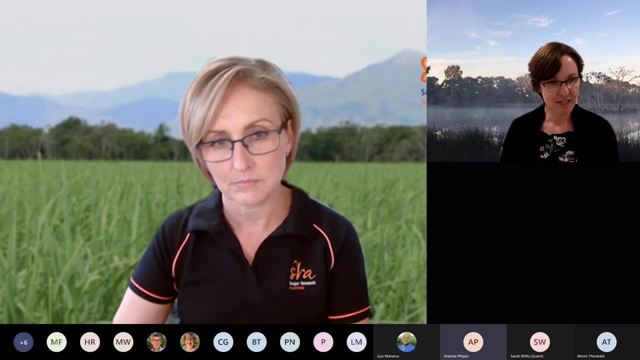 arsenal to be able to actually um, you know, help us. um, i think is good um. you know there clearly are challenges with forecasts on seasonal time scales. it's not an easy thing to forecast um and um and you know it's also. it's also hard to understand probabilities and that sort of. 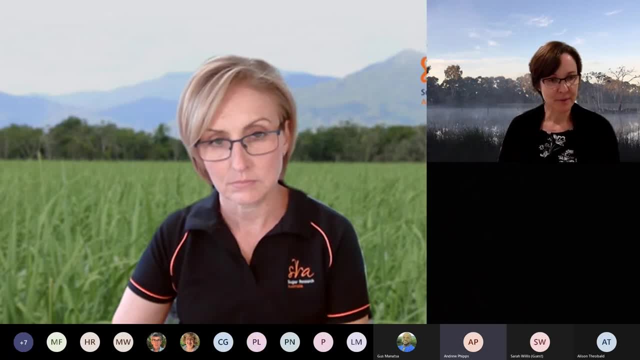 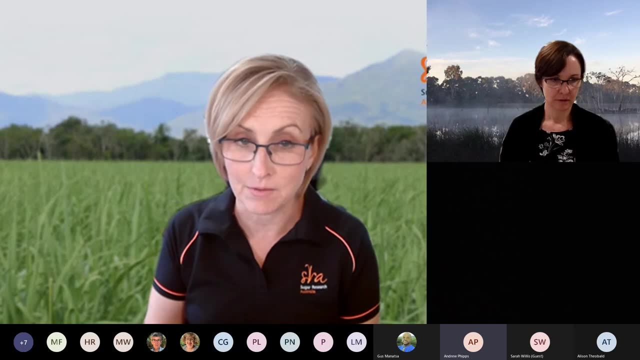 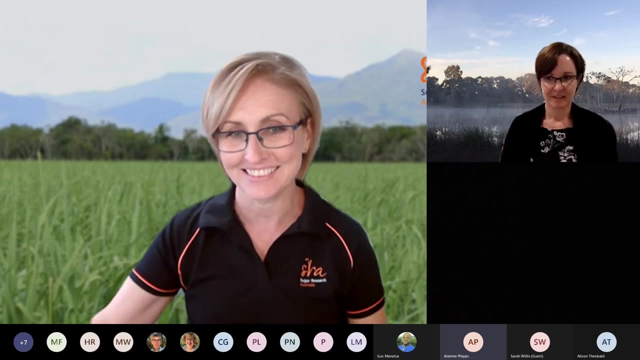 thing, so, um. so there's a lot of. i think there's a lot of progress we can make in terms of of um making forecast more useful, but certainly any information um has to help right as, as the project says, being forewarned is is for armed, you can actually make decisions, yep. 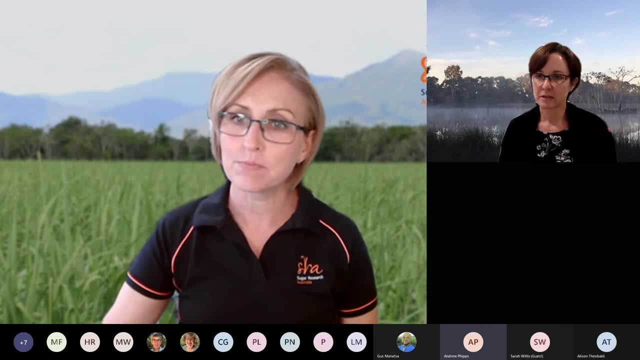 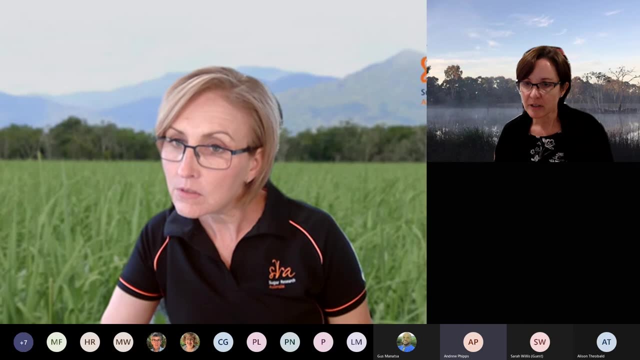 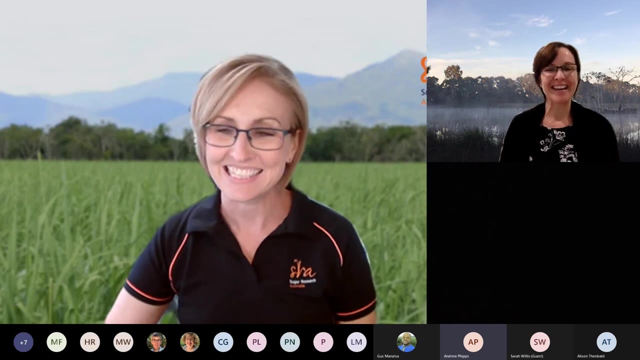 okay, well, look, um, we're not seeing um a whole. a whole lot of other questions come through. I think this is the one there, Cathy, from Luciano, How does the ensemble size affect the predictions? That's a really good question. So, basically, the bigger your ensemble size, the better. 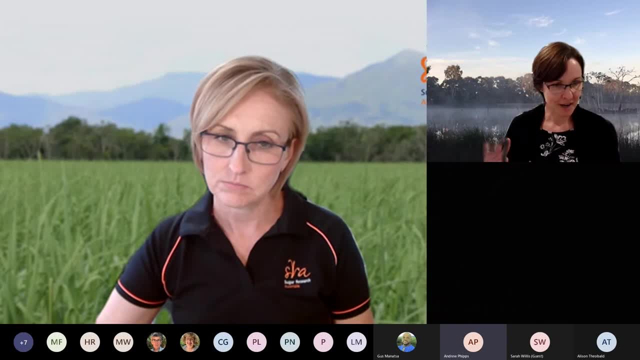 and that does saturate. So you probably don't need more than like 100, but there's a big difference between having 100 and only having, say, five, because basically, the larger your ensemble size, the more options you're considering. 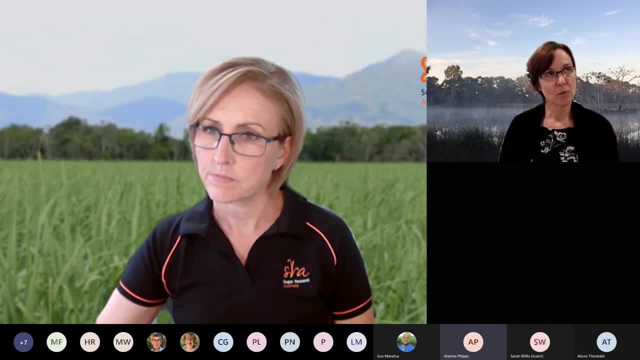 And it's also so, basically, the way that we produce the ensemble takes into account certain amounts of uncertainties that we have. So we have uncertainties in terms of that initial state. when we start the forecast, We don't obviously know what the ocean is going to look like. 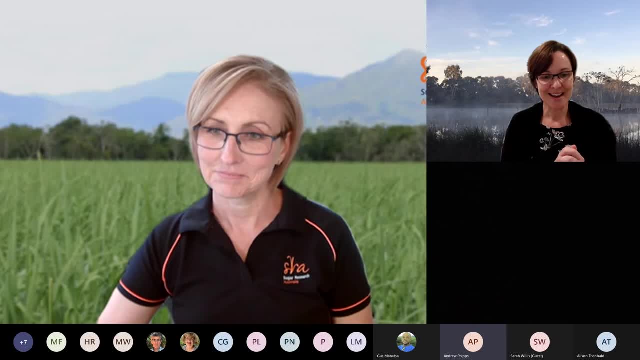 We don't know what the ocean is going to look like, We don't know what the temperature is in all regions of the ocean, or we don't know at every point in the globe and up into the atmosphere. So we have uncertainties in that initial state. 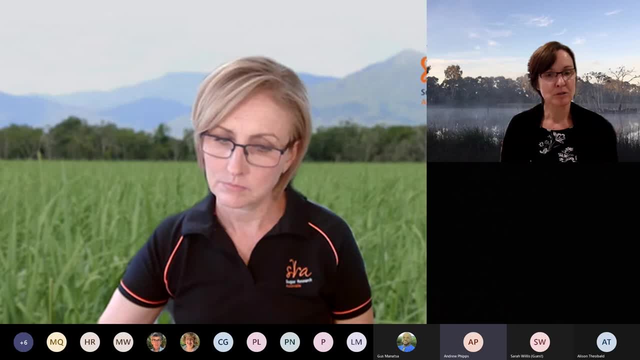 and so we take that into account. And then this is a model, and the model is not perfect, So we have uncertainties associated with the actual model, And so taking that into account is important as well, And that's why it's often useful to – that's why we also look. 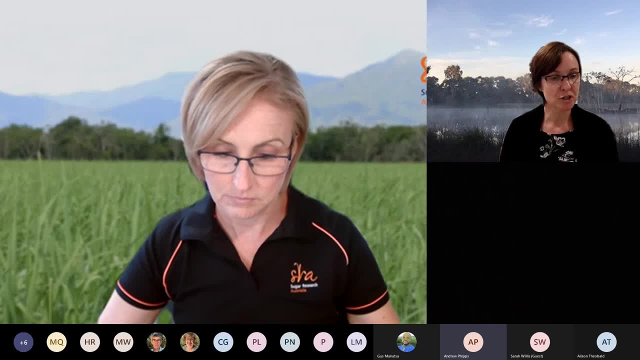 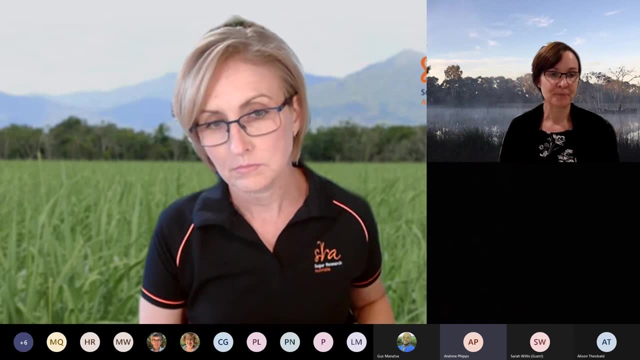 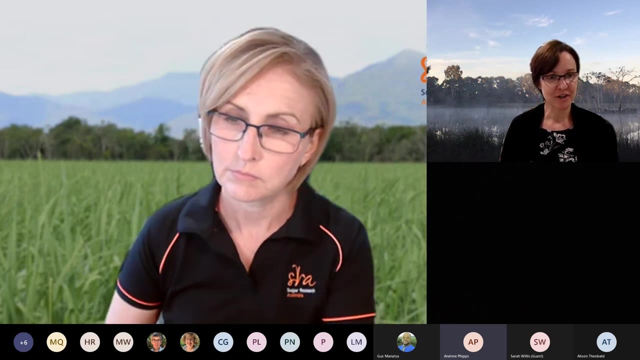 and see what other models are forecasting. So we'll look and see. We'll look and see what other international models are forecasting and see you know how much agreement is there between those models. So ensemble size is a very important consideration. Another point about that is that it's very expensive. 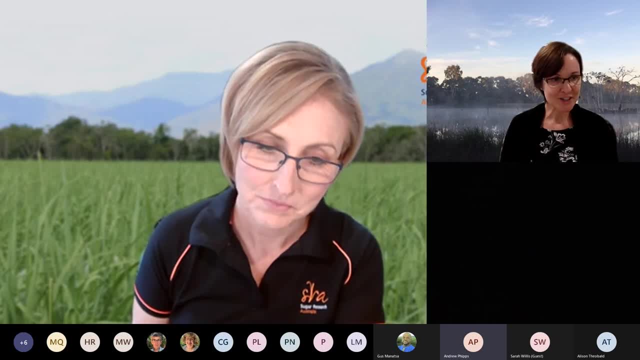 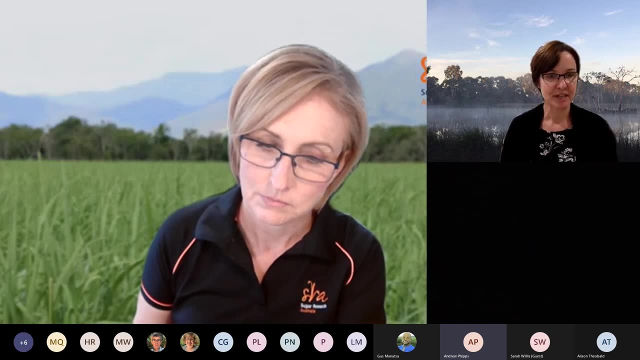 to run these models. We run them on a supercomputer, So we're always trying to balance out, you know, how much can we afford to run, How much can we spend on the supercomputer, And so a lot of the stuff is constrained. 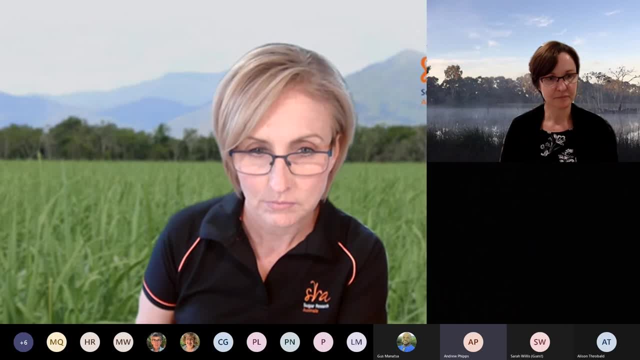 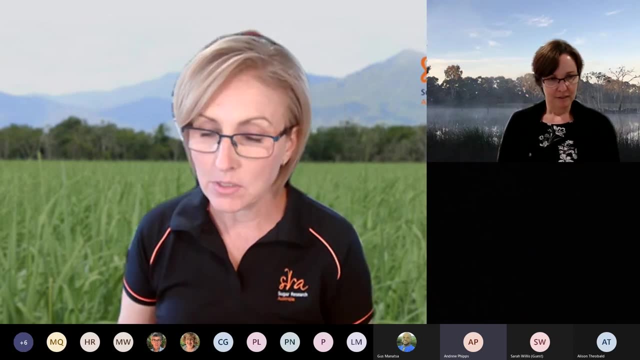 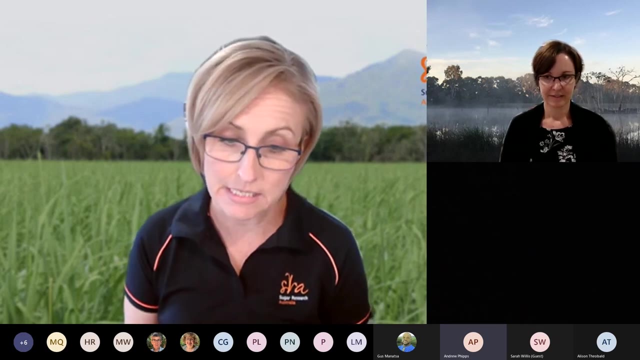 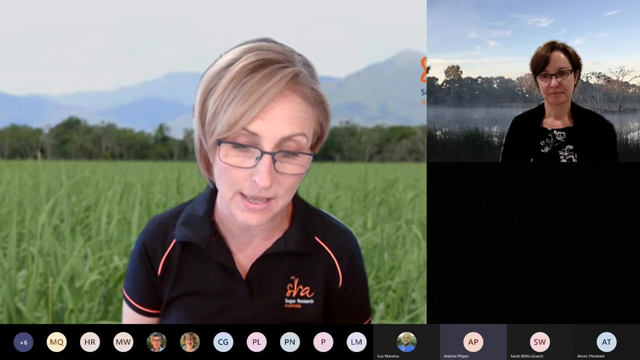 by supercomputer availability. Thank you Well, Debbie. we might look to wrap up there. Can I say a big thanks to you for sharing your expertise with us today. We're certainly very grateful for your time and your knowledge and I do hope that those on the call have found it useful. 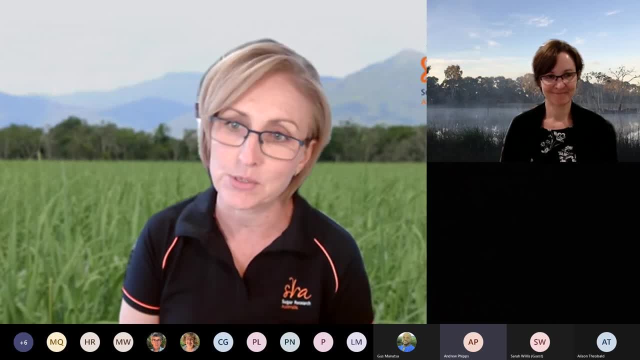 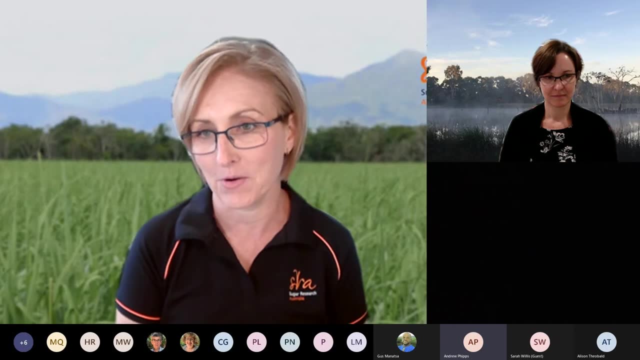 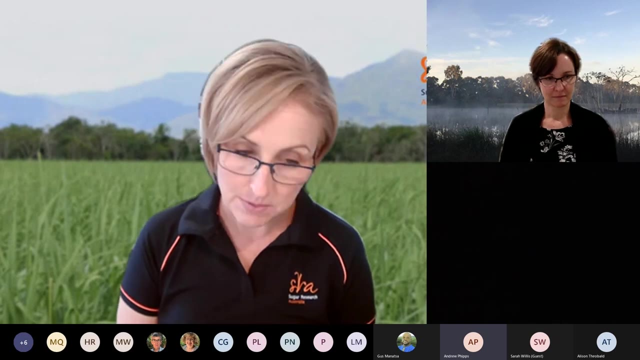 I can see that Sam has acknowledged a great presentation on a complex issue with a lot of variables to consider and noting that the tools are very important for all and for the future. So thank you, Look, we would love to hear your feedback more formally too. 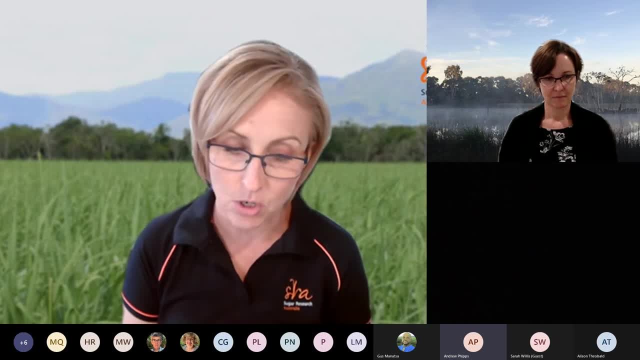 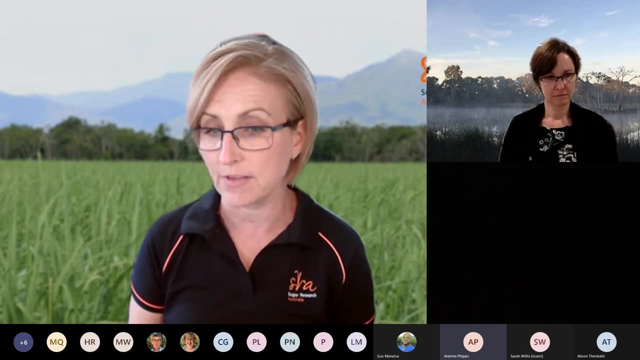 please about today's session and ask if you can please take a few moments to complete the feedback form that I have shared in the chat function. It's a simple online session, Thank you. It's a simple online survey. It won't take more than a couple of moments to complete. 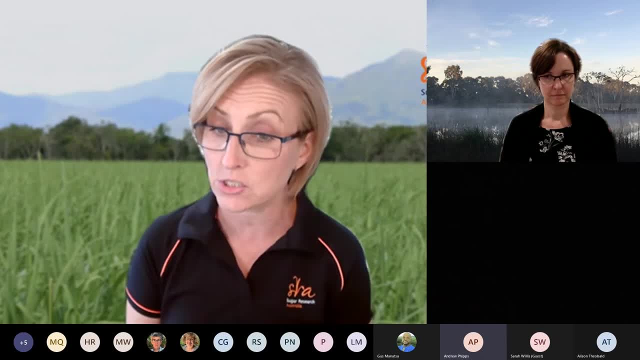 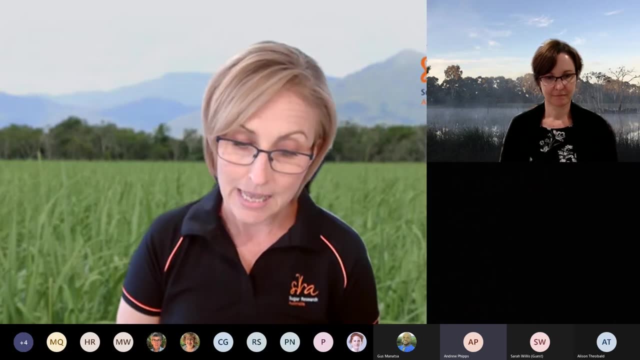 I've also shared my contact details so that, if you have any further questions, please do feel free to reach out and we'll put you in touch with the appropriate people. We do have another webinar scheduled for this Friday, as Debbie mentioned, and it I guess